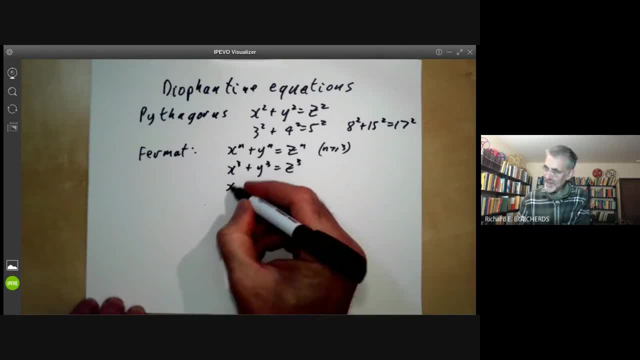 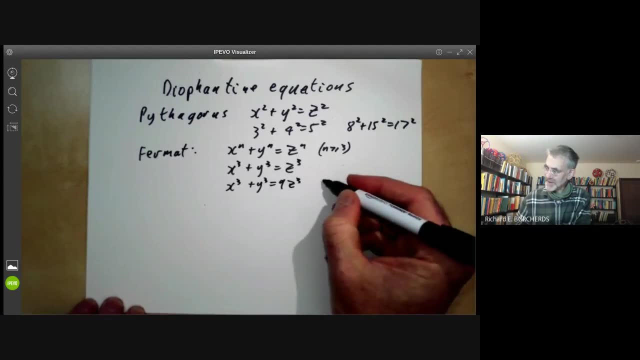 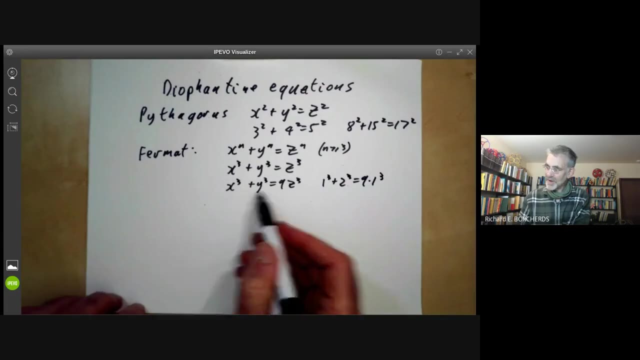 because it's got no solutions to find. So instead we could look at some variation of it like x cubed plus y cubed equals nine z cubed, And this certainly has a solution. one cubed plus two cubed equals nine times one cubed, And we can ask if it has any other. 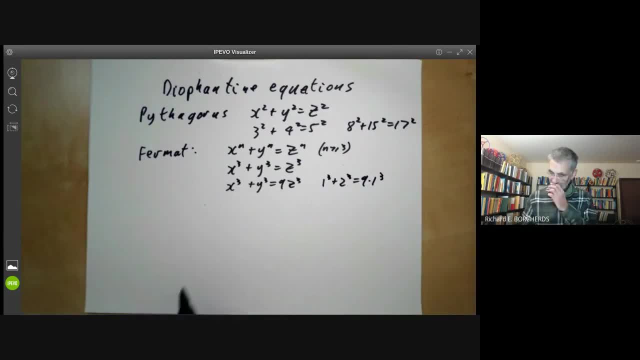 solutions And if so, how do we find them? So another example of an equation with a curve actually has a singularity, as we will see later, is something like y squared equals x squared plus x cubed. So this is a solution: six squared equals three squared plus three. 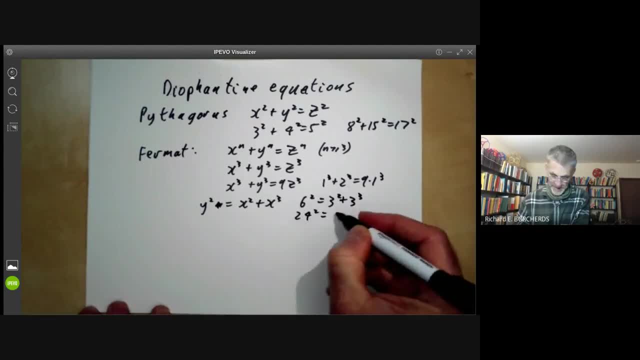 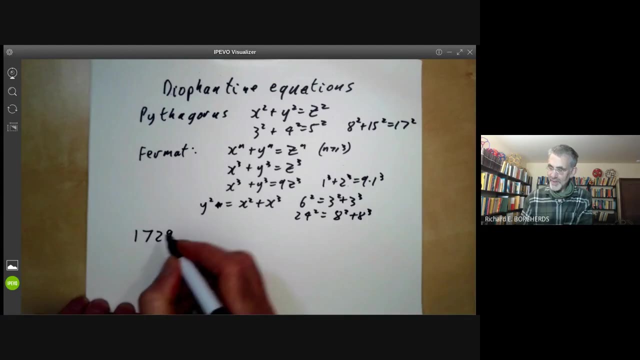 cubed or 24 squared equals eight squared plus eight cubed. And again we can ask: can we find all integer solutions of this? So next example is the number 1729 is fairly famous for a reason- I'll explain a little bit later- And it can be written: 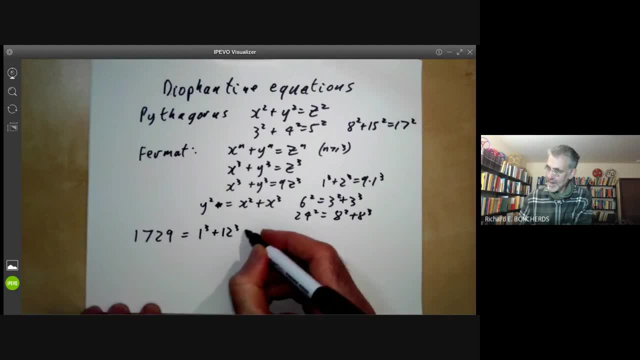 as a sum of two cubes in two different ways. So you can ask: are there other numbers that can be written as a sum of two cubes in two different ways? So we're trying to solve w cubed plus x cubed equals y cubed plus z cubed. 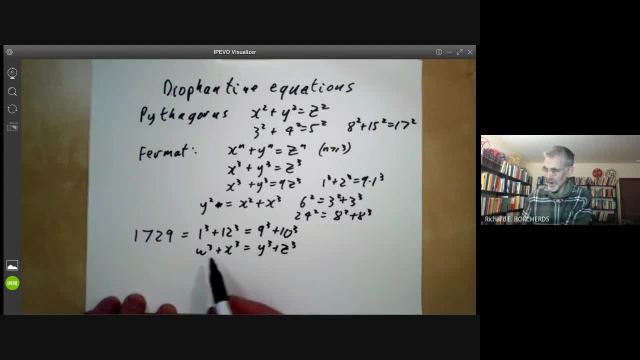 And there are some trivial solutions where w is equal to y or w is minus x or whatever. So we want to find non-trivial solutions of this. For example, we could have two cubed plus 16 cubed equals nine cubed plus 15 cubed, And again we can ask: how can we find solutions of this? Well, 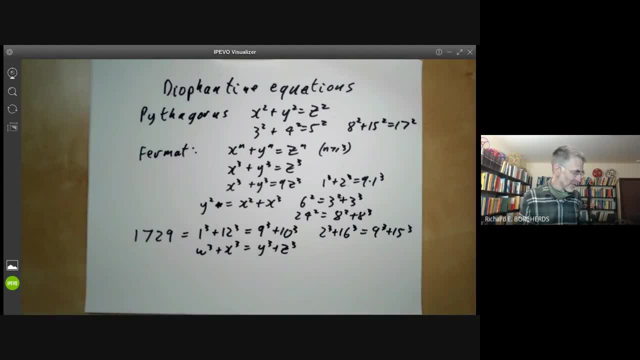 one way to find solutions of all these equations is just a kind of stupid one. We could just get a big computer and have it checking every possible case, And this would sort of very slowly find solutions like this. But what we want is a, is a sort 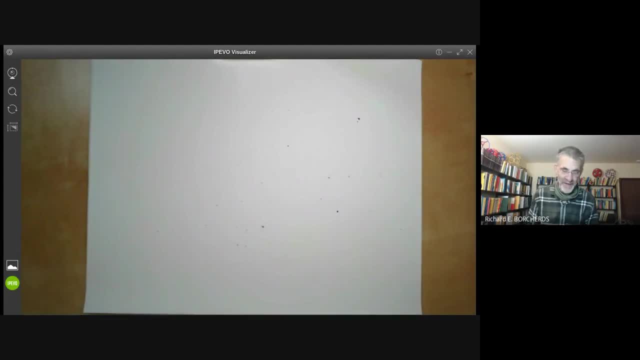 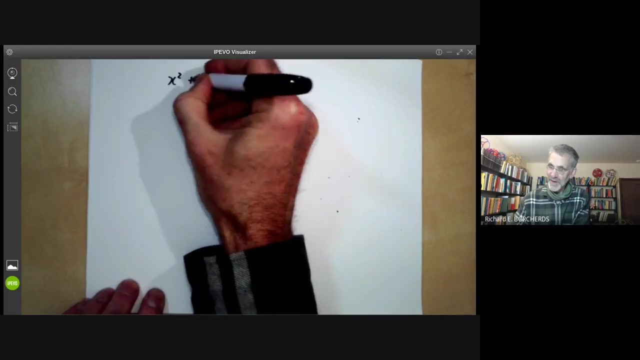 a lazier way of finding solutions with less effort, And what I'm going to do is show how to find solutions of Diophantine equations by using geometry, And the geometry makes it much easier to find solutions. So let's look at the first example- Pythagoras equation- And we can divide it by z squared. 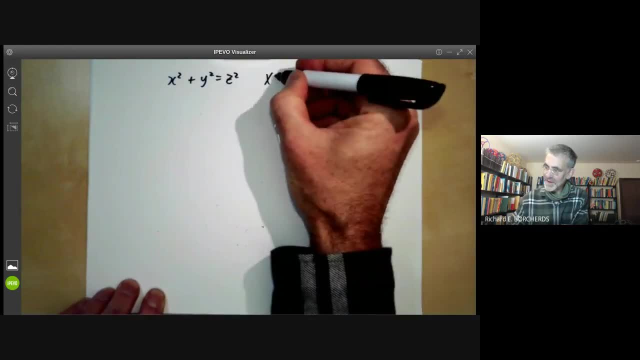 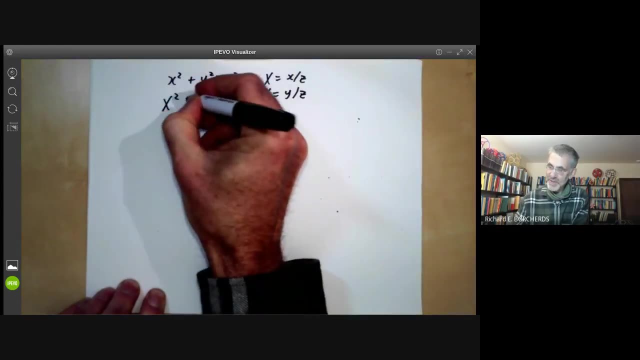 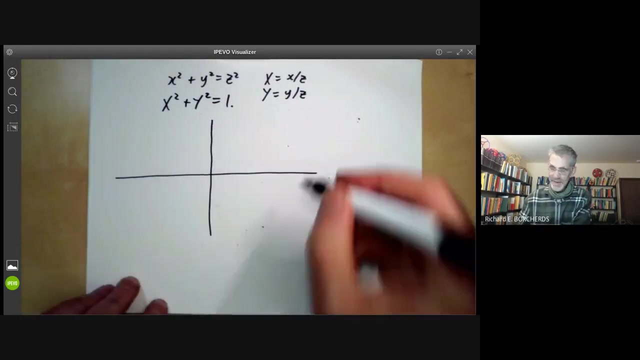 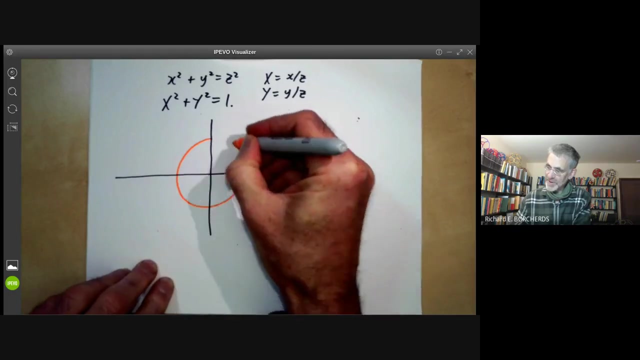 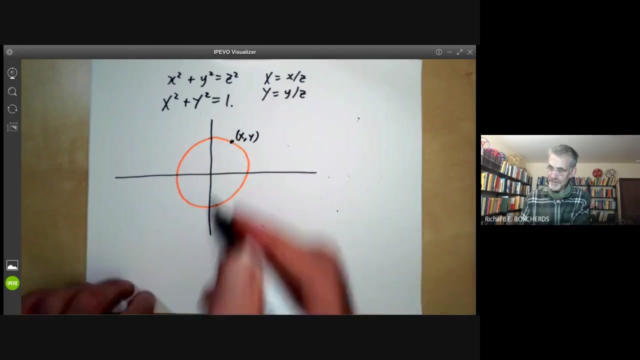 right, Okay. So if I put x equals x over z, y equals y over z, then this equation becomes x squared plus y squared equals one, And you can recognise this as the equation of a circle. So what we're trying to do is to find points on the circle with rational coordinates. 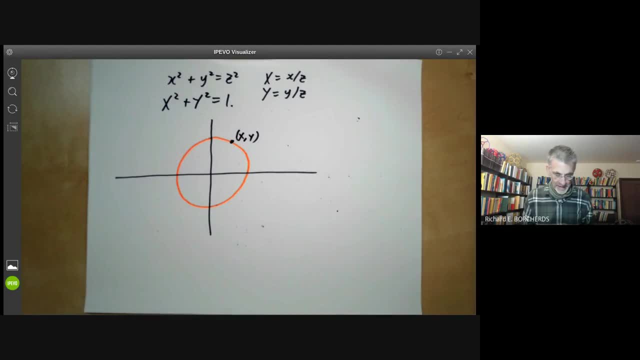 So how can we find those systematically? Well, what you can do is there's an obvious point with rational coordinates, which is this one, and I guess, these four here, which just as coordinates minus one zero. And what I'm going to do is I'm going to just draw a line through these two. 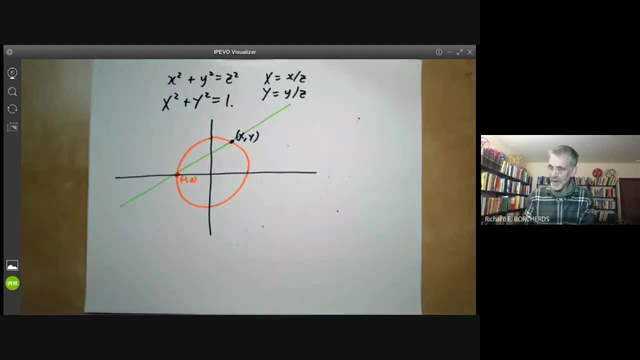 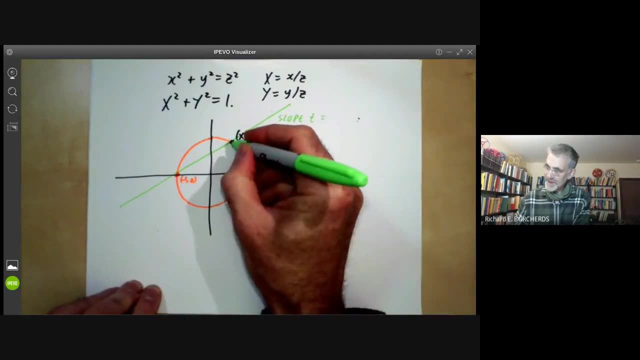 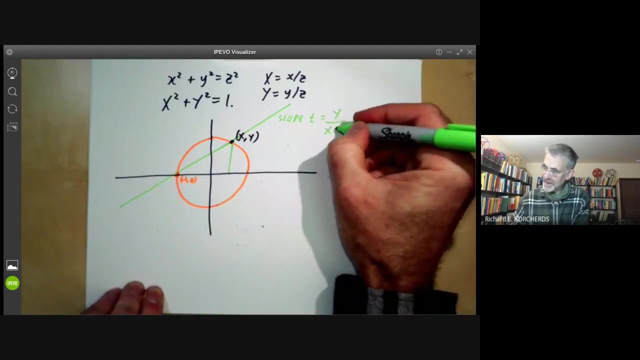 I'm just going to draw a straight line through these, And this straight line has a slope. It's called the slope t, And the slope t is easy to figure out. It's just this distance here divided by this distance here, which is just y over x plus one. 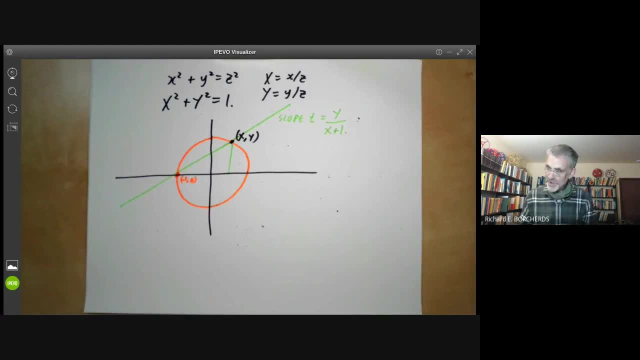 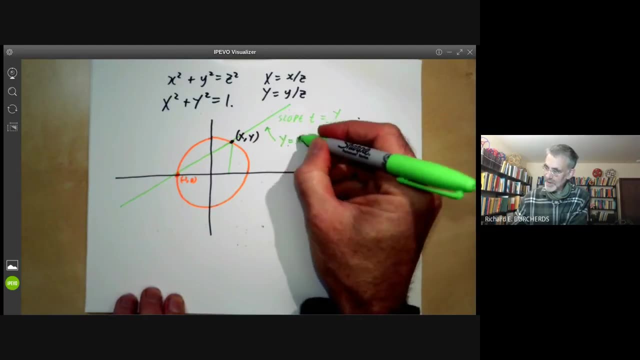 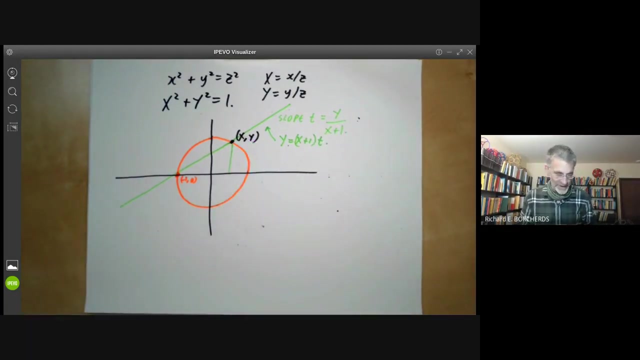 And now we can work out the equation of this line. So this line is just the line y. So y equals x plus one times t. Now you notice, t is obviously rational if x and y are rational. So we can say x, y rational implies t is rational. 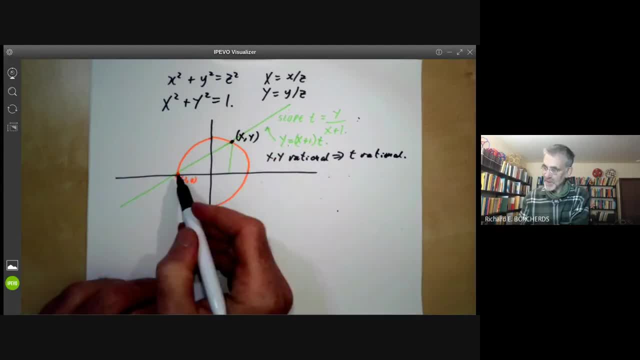 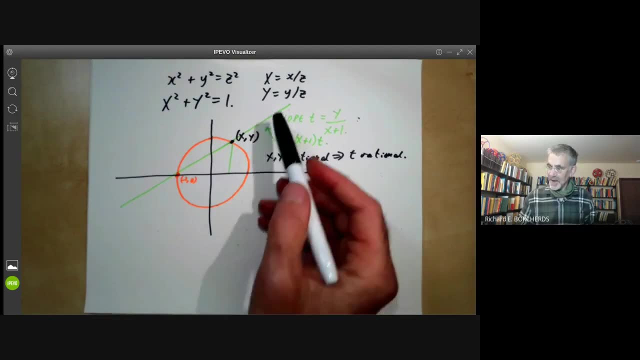 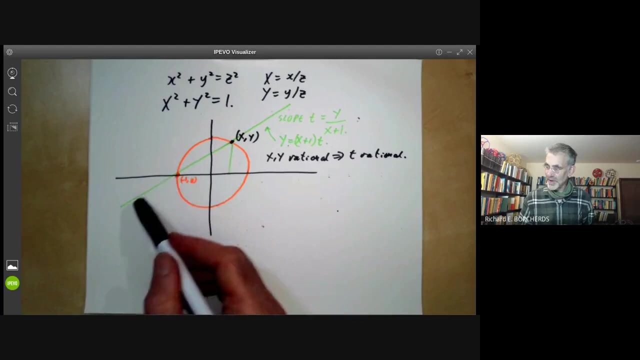 And we can ask the converse: if t is rational, are x and y rational? And you can see the answer is yes, without doing any calculations, as follows: Because this circle has a degree two equation. So if you try and find the intersection points, 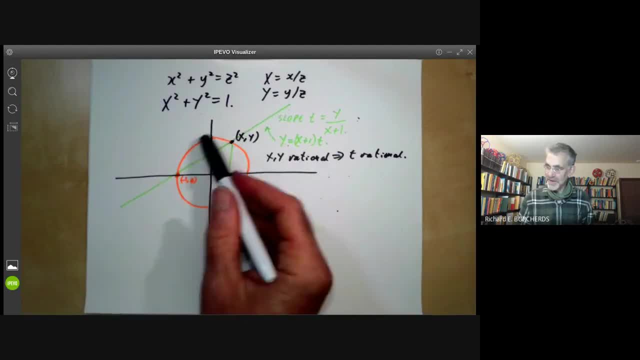 suppose you try and find the x coordinates of the intersection points of a line and a circle, there'll be two intersection points, which is the solution of some quadratic equation. This quadratic equation has rational coefficients And we know one of the roots is rational. 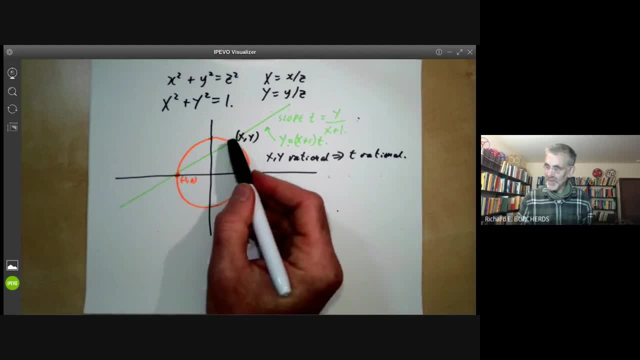 So the other root must be rational, because the sum of the roots of a quadratic equation with rational coefficients is rational. So we know, before we do any calculations, that if we pick a rational t, then x and y will be rational. Well, now let's actually calculate them. 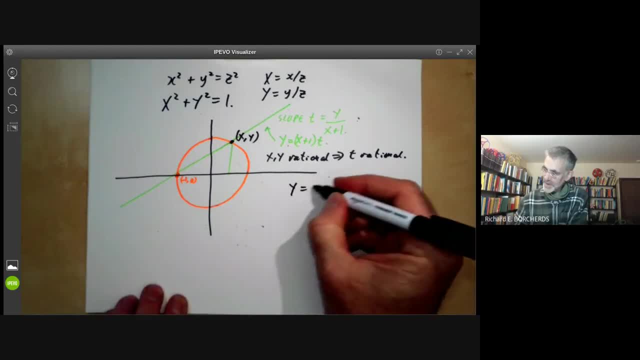 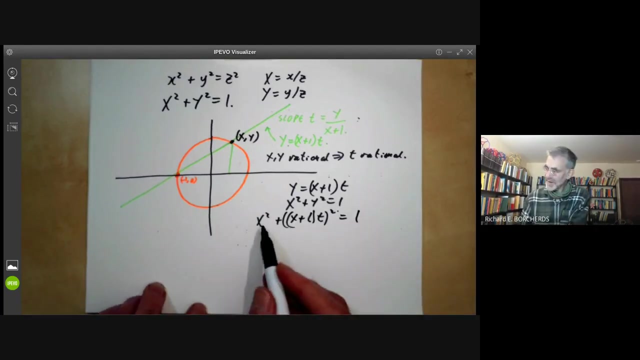 So we have y equals x plus one times t. And we also know x squared plus y squared equals one. And if we substitute y into here, we find x squared plus x plus one times t. t all squared is equal to one. And now this is a quadratic equation in x. 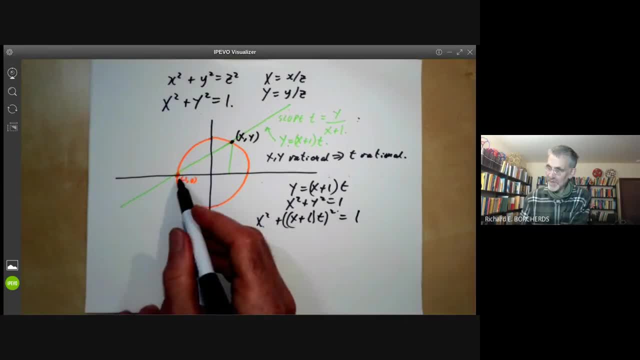 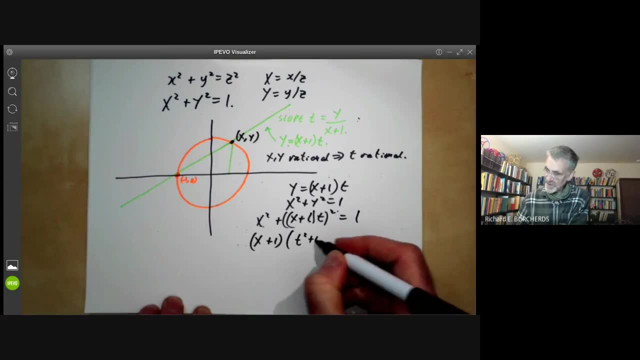 So it has two roots And one of the roots is minus one. So it must factorize as x plus one times something And you can work out what the something else is. It's t squared plus one times x plus t squared minus one equals zero. 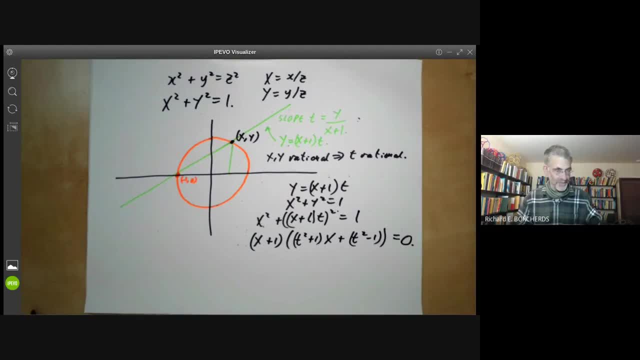 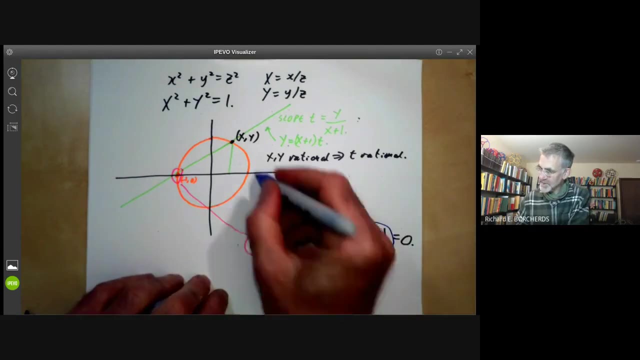 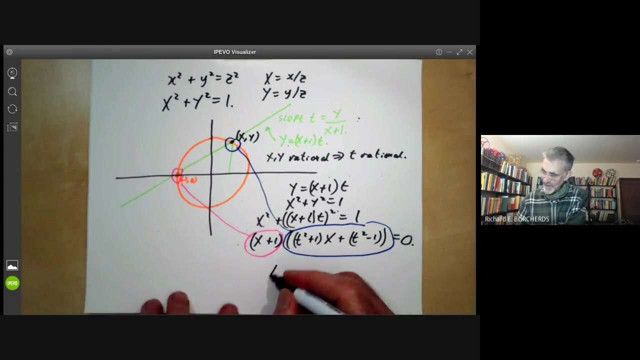 So here's the root: x equals minus one, which corresponds to this point here, And here is the other root, which corresponds to this point here. And you see, we can work out what x is We have. x is equal to one minus t squared over one plus t squared. 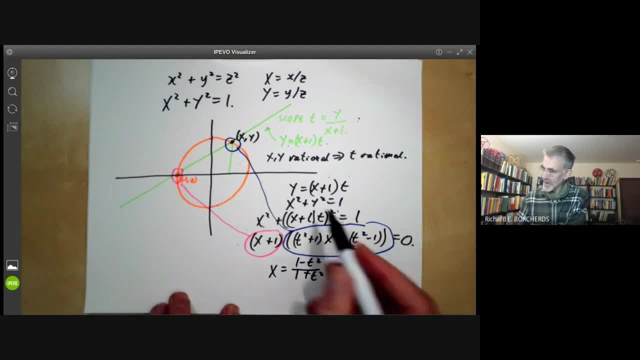 And y is equal to x plus one times t, which is two t over one plus t squared. So you can check by algebra now that if t is rational, then x and y are rational. But these are slightly complicated expressions And we could have found that x 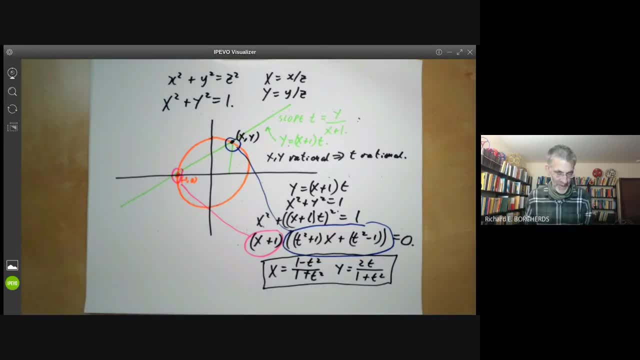 as we said, we don't need to do this calculation to see that x and y are rational. Anyway, we can now find lots and lots of solutions to Pythagoras's equation, Just by choosing t, For instance. if we choose, t equals a half. 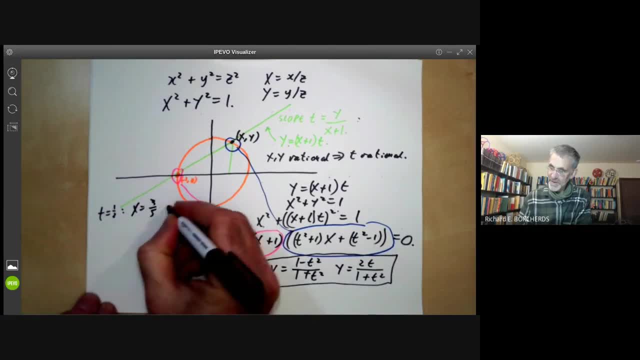 we find x equals three fifths and y equals four fifths, which gives us the equation: three squared plus four squared equals five squared. If we choose t equals- let's just choose any random rational number- three over 11,. we find x is equal to 56 over 65,. 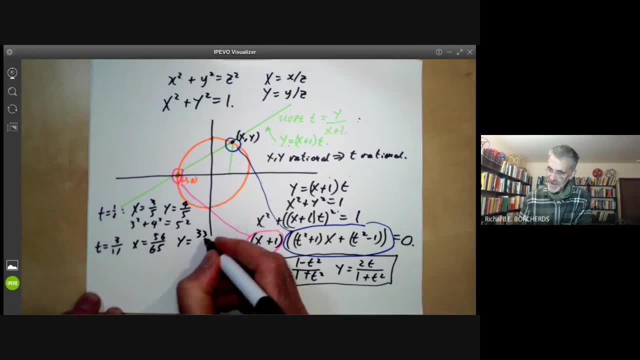 and y is equal to 35.. If we choose t equal to 33 over 65, giving us the solution 56 squared plus 33 squared equals 65 squared, And you can obviously generate effortlessly generate enormous numbers of solutions to this just by picking a rational number: t. 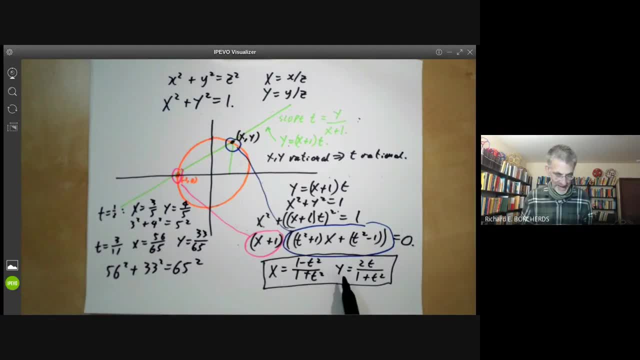 and working out x and y from that. So this actually gives essentially all solutions of this equation, because solutions of this equation more or less correspond to rational numbers t. There's one slight exception: This point here doesn't correspond to a rational number t. 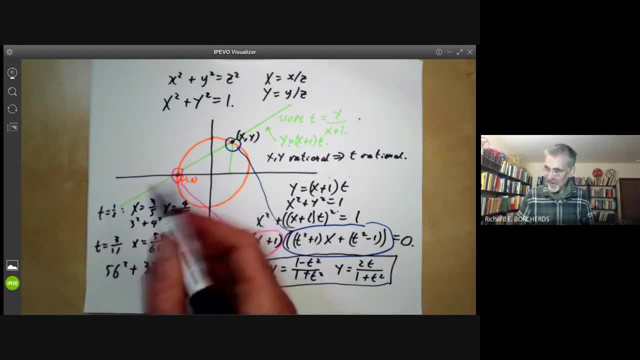 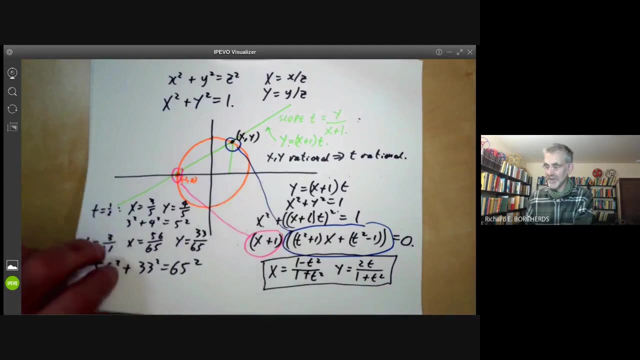 It corresponds to the point: t equals infinity. But apart from that we get a one-to-one correspondence between solutions of this and rational numbers. So we've got a complete description of the solutions. So that's one geometric way of finding solutions. There's actually a second geometric way. 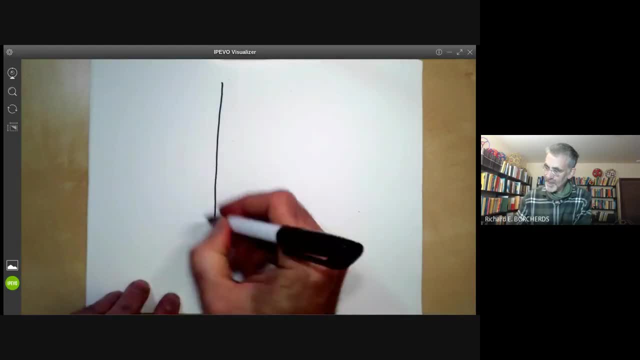 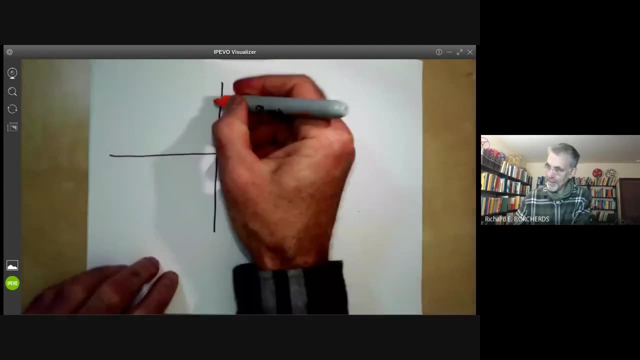 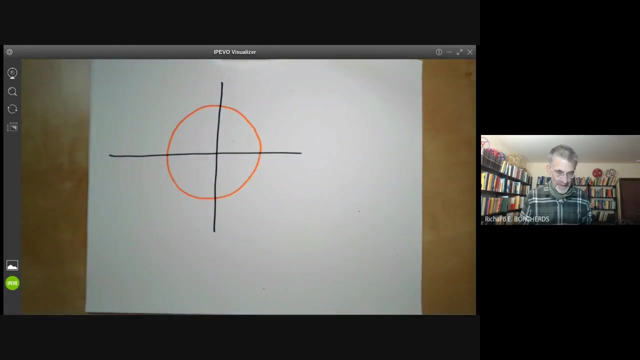 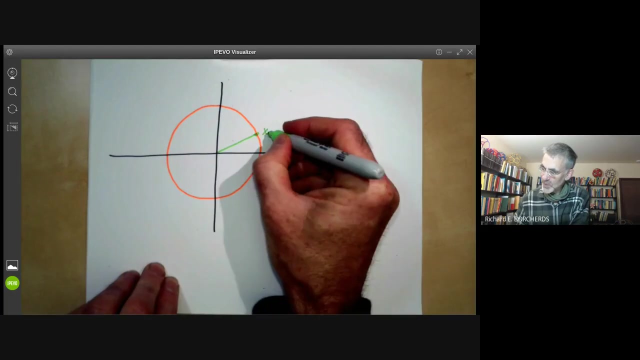 of finding solutions of this. So we again draw a circle Like so, And this time let's write down a solution. Yes, suppose you've got some point: x1, y1. And let's just look at this angle: theta. 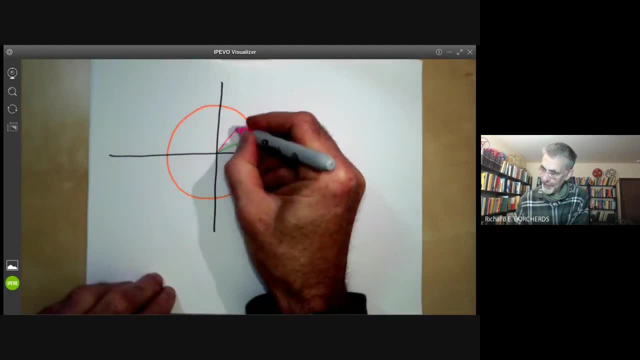 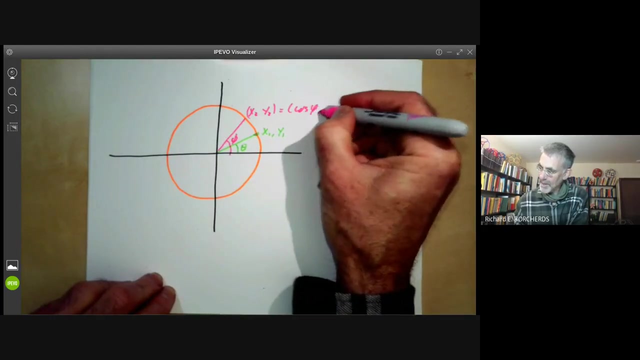 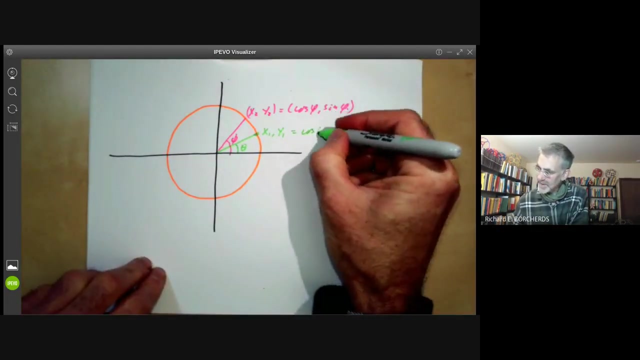 And suppose we take another solution And let's call this angle phi. So here we're going to have a solution: x2, y2.. And you can see, this is equal to cosine phi sine phi. And this one is of course equal to cosine theta sine theta. 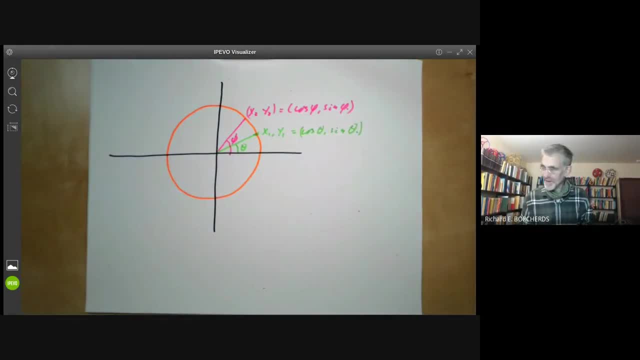 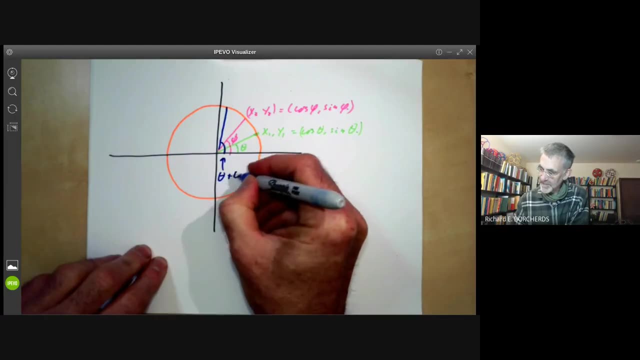 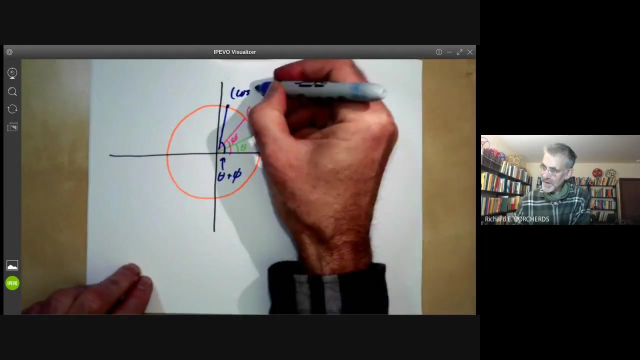 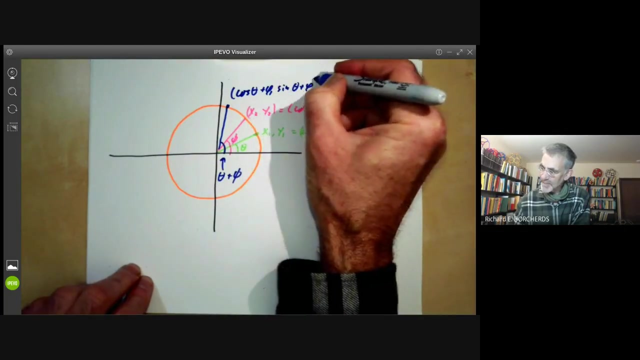 And now what I'm going to do is I'm just going to add up theta and phi. So now I'm going to have this angle: here is going to be theta plus phi, And the coordinates of this point will be cosine theta plus phi, sine theta plus phi. 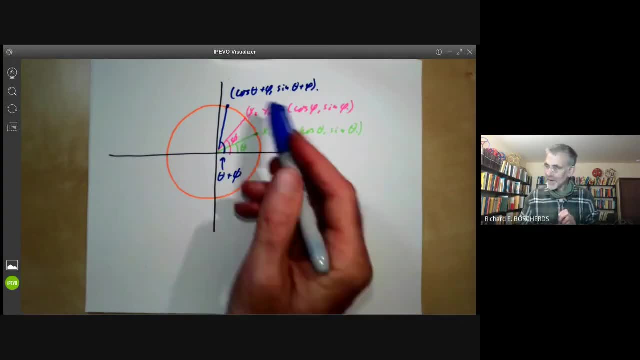 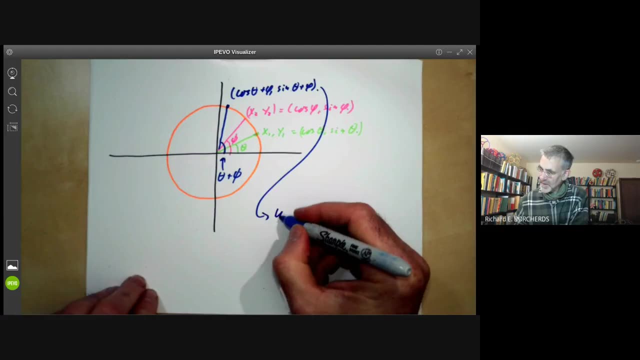 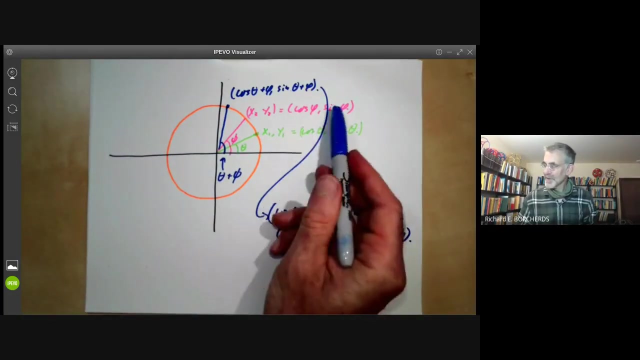 And now we can use the formulas for the sum of two angles. So this root here will just be cosine theta cosine phi minus sine theta sine phi. And then we have cosine theta sine phi plus sine theta cosine phi. And now what you notice from this is that if all these numbers here are rational, 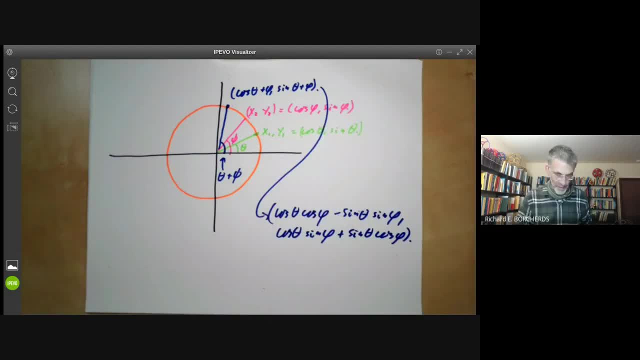 then these numbers here are also rational. So what this means is, if we've got a solution x1, y1 and a solution x2, y2 of Pythagoras' equation, then we can find a new solution as follows: So we've got x1, y1, with x1 squared plus y1 squared equals 1.. 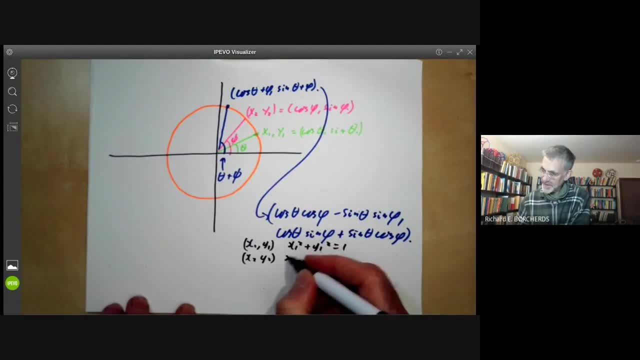 And we've got x2, y2, with x2 squared plus y2 squared equals 1.. And now we take this point here, which is the point x1, x2.. minus y1, y2, x1, y2 plus x2, y1.. 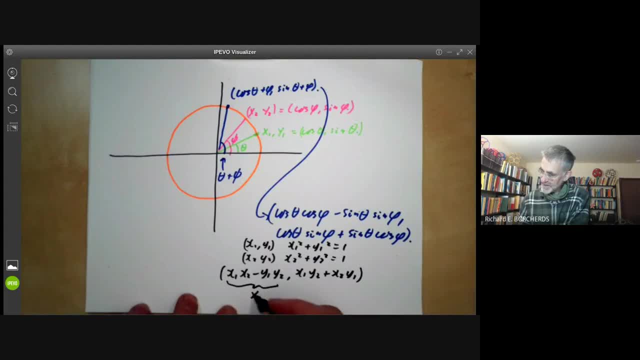 And if we call this x and this y, then we see that x squared plus y squared will also be 1.. So this gives a way of generating new solutions from old solutions using this formula. Notice that algebraically this formula is a bit mysterious. 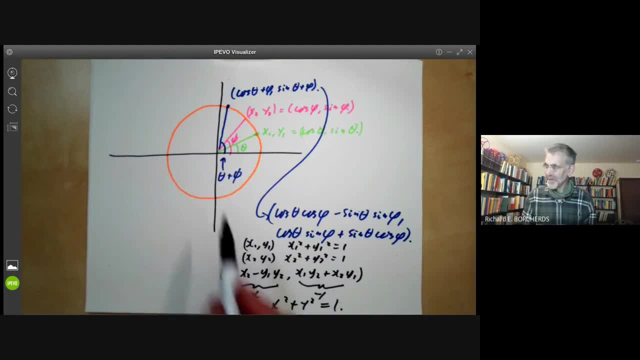 It's not something you would immediately think of, But if you think of it geometrically, it's obvious what's going on. You're just adding up two angles. For example, we had a solution: 3 fifths, 4 fifths. 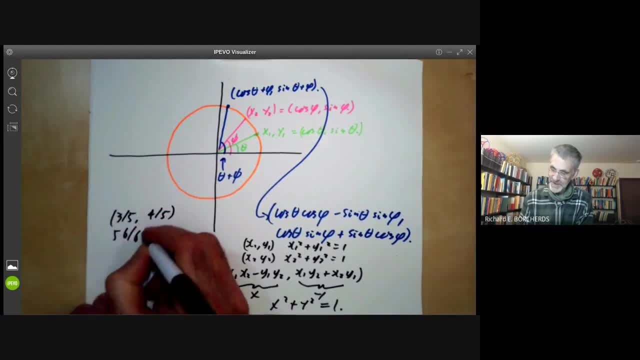 And we had another solution: 56 over 65,, 33 over 65.. And if we take this to be x1, y1 and this to be x2, y2, we can work out this equation here, And it turns out to be 36 over 325. 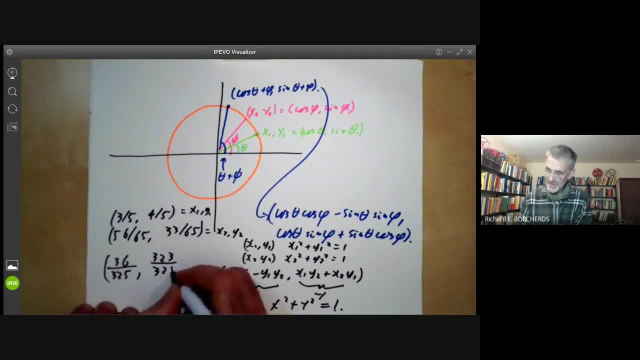 323 over 325.. 323 over 325.. So we found another solution of Pythagoras' equation: 36 squared plus 323 squared equals 325 squared. And we can obviously carry on doing this and produce more and more, larger and larger solutions. 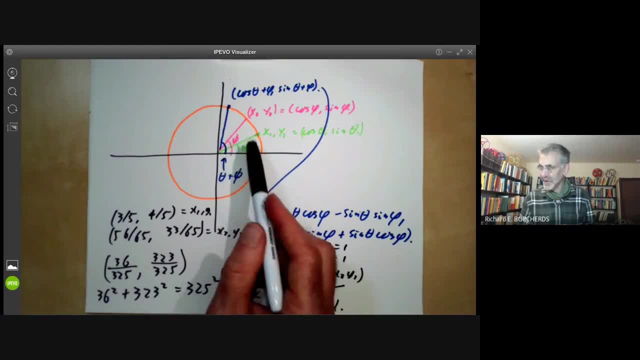 Incidentally, this shows that the solutions of Pythagoras' equation form a group, which means we can sort of there's a sort of way of adding up two solutions to get a third solution. So here we take this solution and this solution. 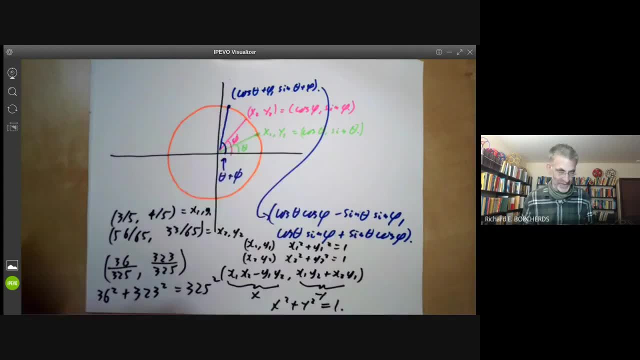 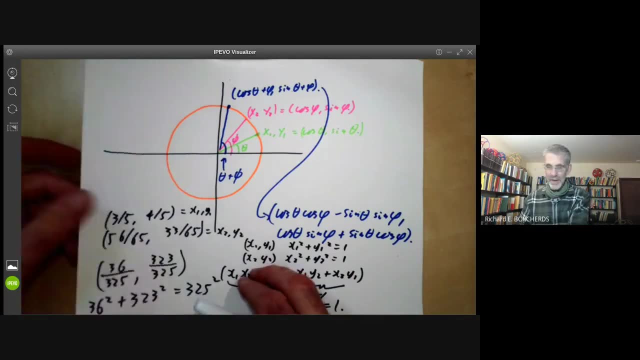 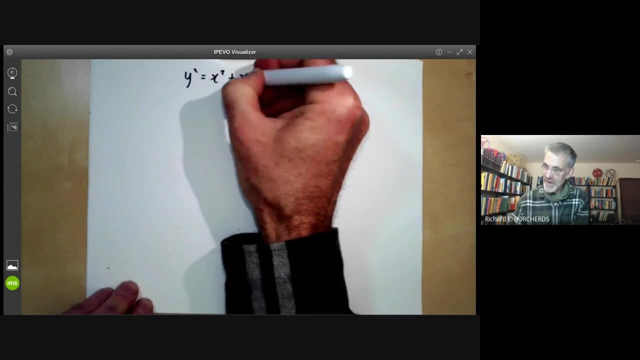 and sort of add them together to get that solution. OK, now let's look at another equation. So let's look at the equation y squared equals x squared plus x cubed. So we have solution: 6 squared equals 3 squared plus 3 cubed, for example: 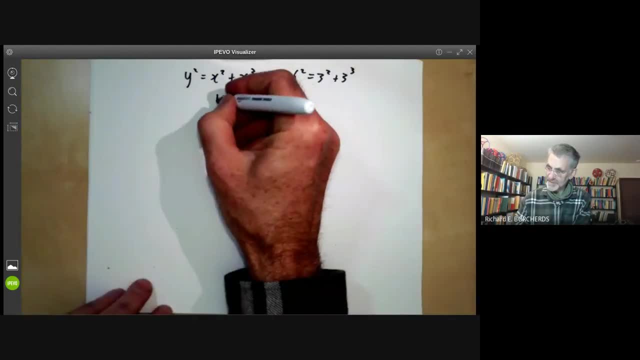 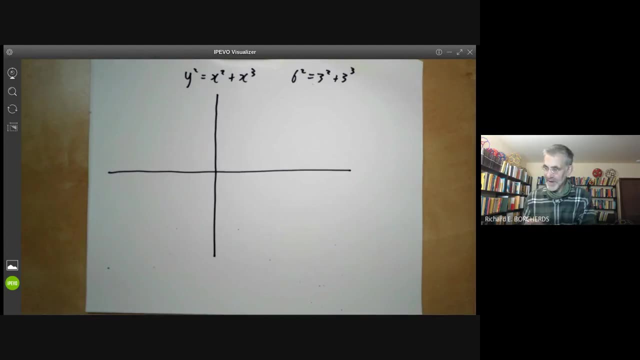 And we want to find all solutions And we're going to do it geometrically. So let's draw a graph of y squared equals x squared plus x cubed And it looks something like this: You sketch it And you notice there's a sort of funny singular point here. 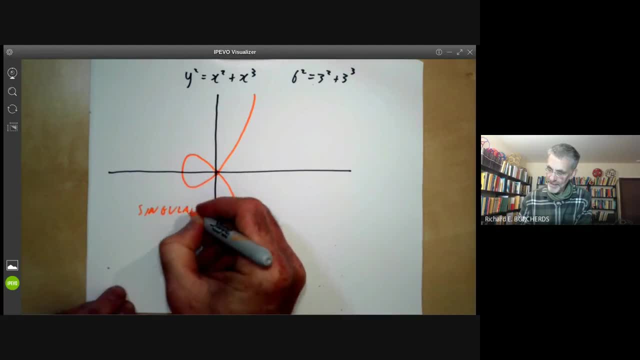 This is called a singularity. So singularity just means a point where things go wrong. So here we've got two. the curve is sort of crossing itself. And also notice there's one obvious solution here: minus 1, 0,. 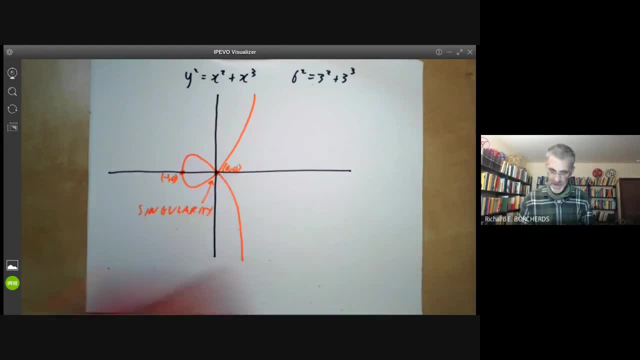 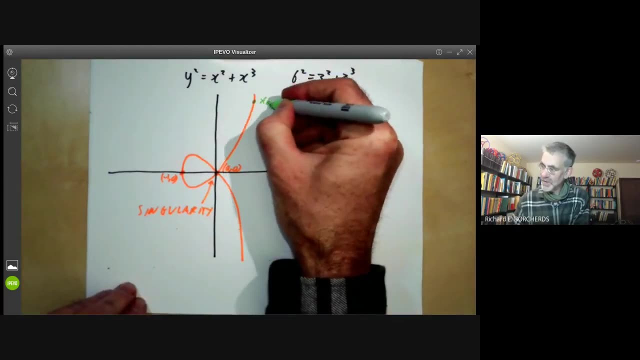 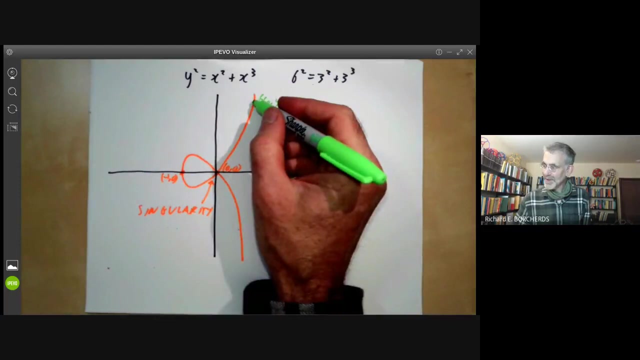 as well as the solution 0,, 0. And now suppose you've got any other solution. Say, we've got a solution- x naught, y naught. Well, what can we do with it? Well, what I'm going to do is I'm going to draw a line through this and another point. 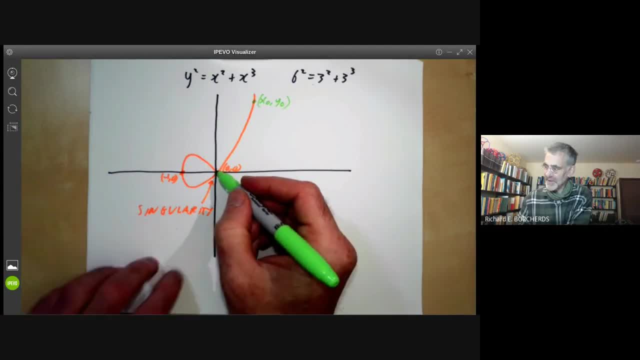 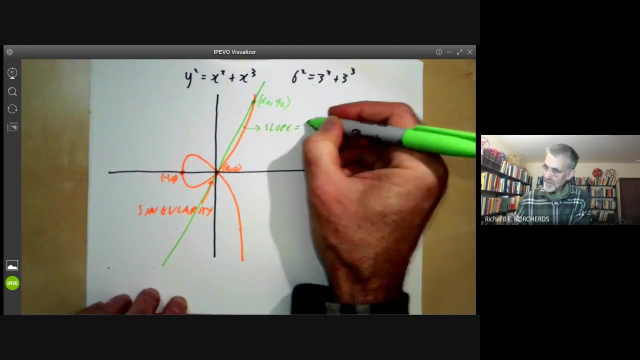 And the most obvious other point to draw the line through is this singularity, because there's obviously something rather special about it. Let's draw the straight line through these two points And let's try and find the equation of this line. Well, it will have. slope is equal to y naught over x naught. 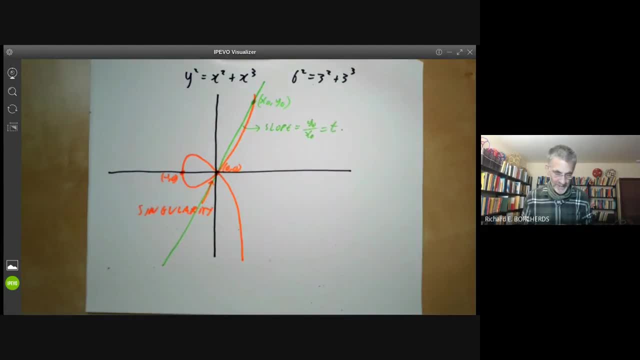 which is equal to t, And this is a cubic equation. So we expect every line, every straight line will generally intersect it in three points. Because if we've got a, if we set y equals ax plus b and substitute it in, we'll get a cubic equation for x. 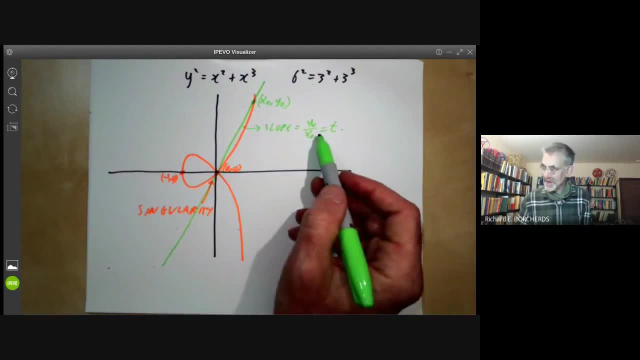 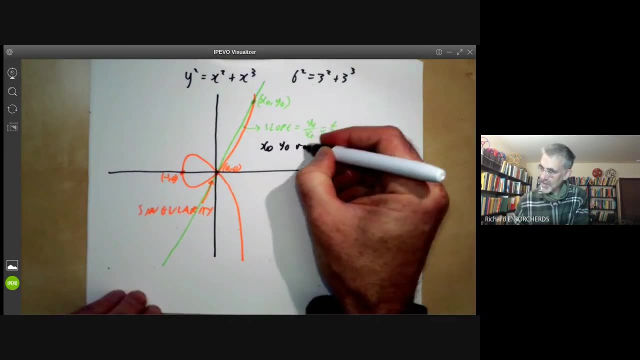 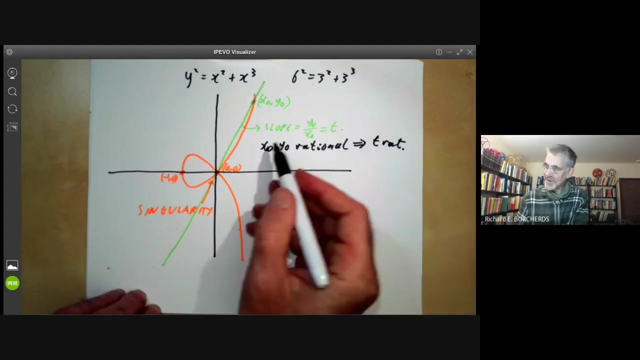 So if x naught and y naught are rational, then obviously t is rational. So let's just note that down. So x naught, y naught, rational implies t is rational. And the question is: if t is rational, does this mean x naught and y naught are rational? 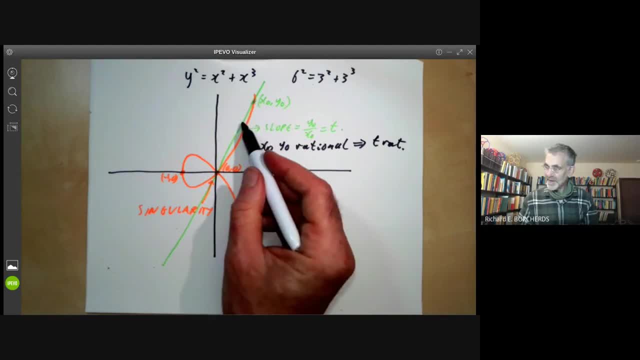 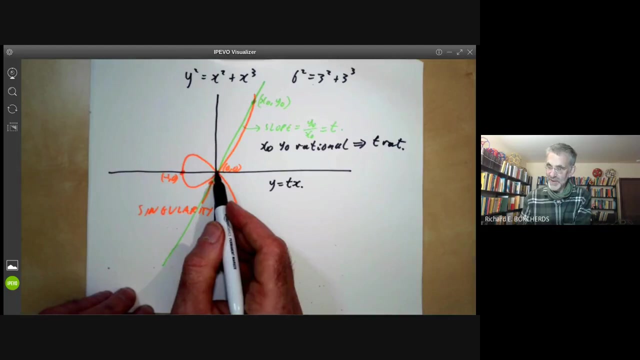 And the answer is yes, because if we fix t, we have the equation y equals tx, And if we substitute this in, we will get a cubic equation for x, And two of the roots are already rational because they're zero. So the third root is also rational. 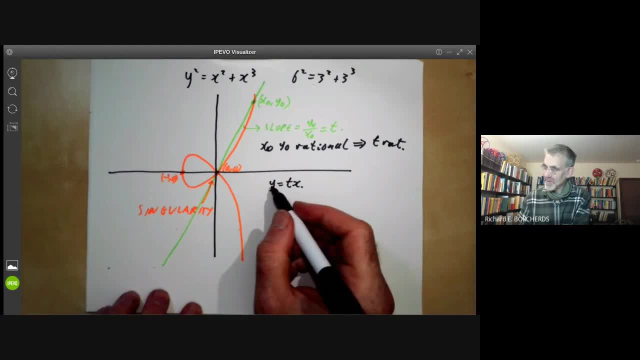 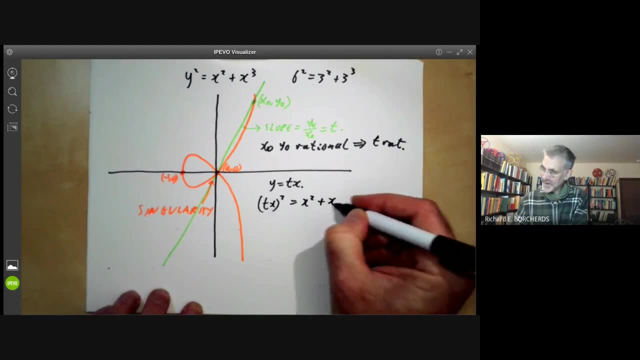 So let's just carry this out. So we substitute: y equals tx and we get tx squared equals x squared plus x cubed. So we have x cubed plus one minus t squared. x squared equals zero. And here we've got a cubic equation. 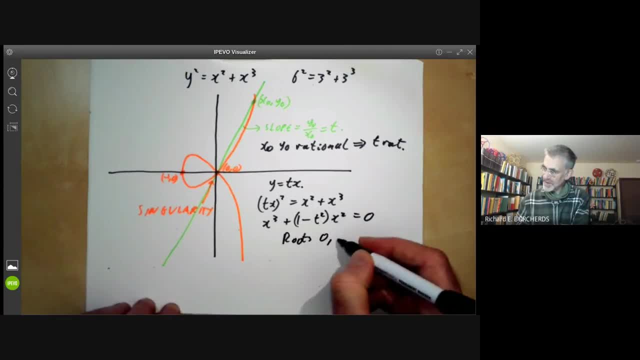 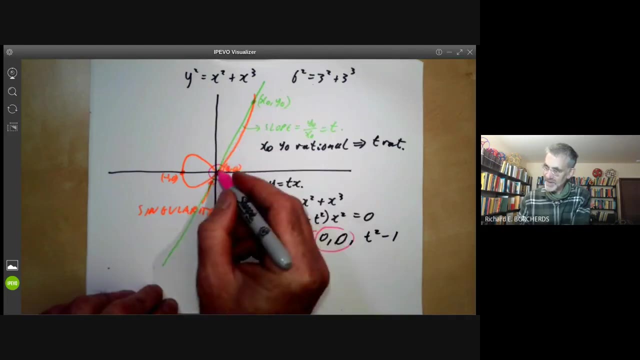 And you can see. the roots are pretty obvious. There's a root zero and zero And the other root is t squared minus one And the two zero roots. you can see them there. They're where this line intersects the orange curve in this double point. 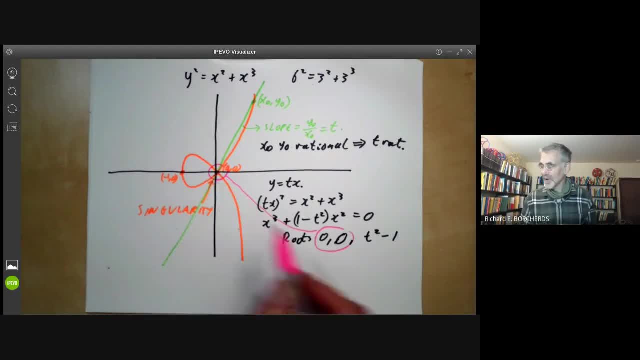 And you see where it's very useful as a double point here, because it means we get two roots that are both zero. So now we can solve this equation. We find x naught is equal to t squared minus one, And y naught is equal to t times x naught. 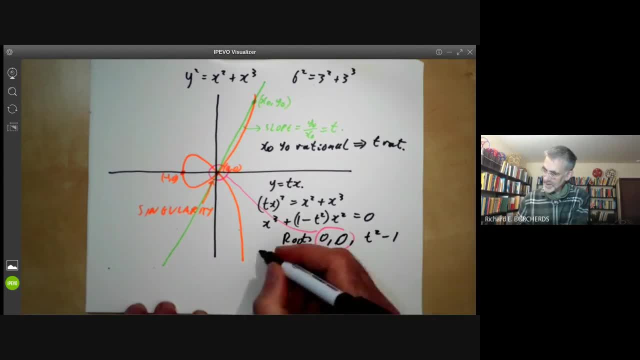 which is t times t squared minus one. So here's a way of finding solutions to this equation: just by writing down rational numbers. And of course you want integer solutions. So we might take t to be an integer, For instance. we could take t equals four. 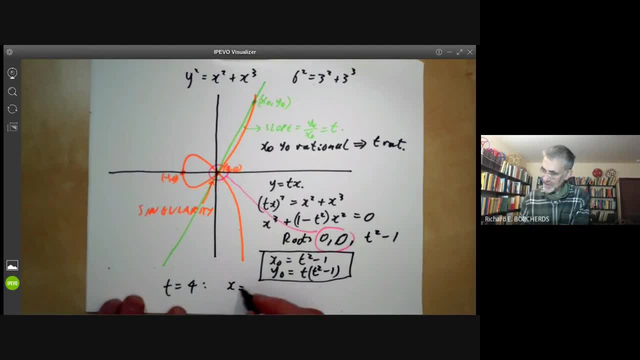 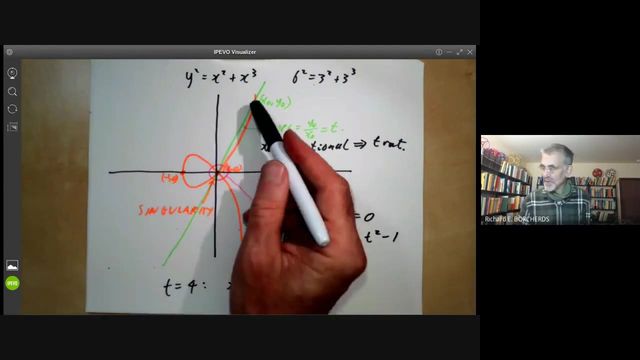 and we get the solution: x equals 15, y equals 60. And similarly, you can generate as many solutions as you like. Well, that cubic equation was particularly easy because it had a double point. What happens if you get a cubic equation? 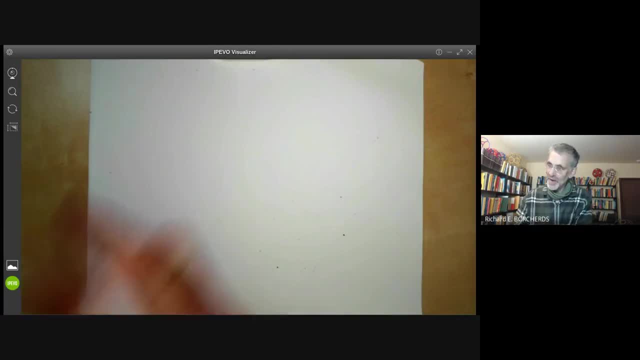 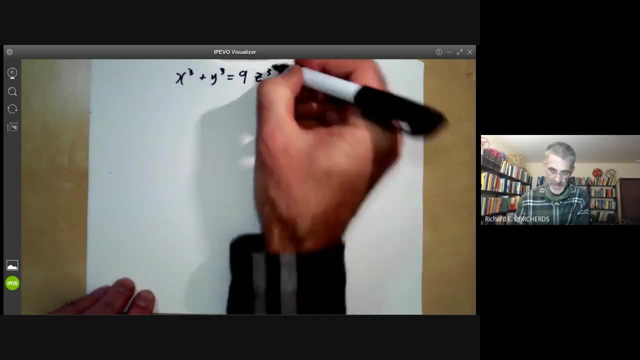 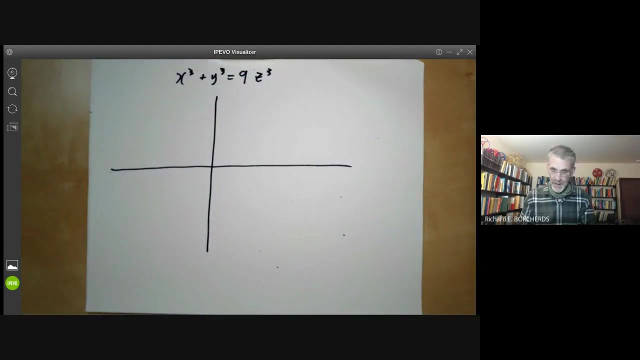 without a double point. So let's try the example I mentioned earlier: x cubed plus y cubed equals nine times z cubed And, as before, let's just sketch this to see what's going on. And it looks something like this: 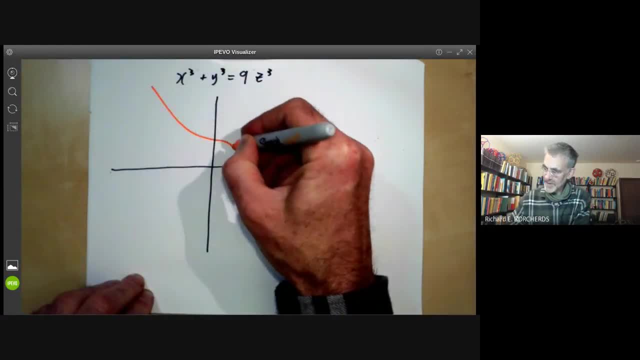 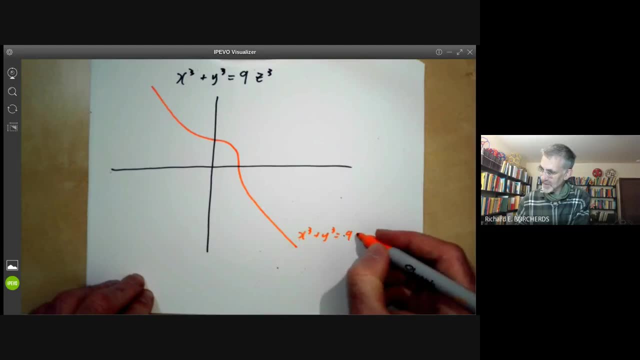 It's got a sort of asymptotic y equals minus x and it ends around like this: So it is x cubed plus y cubed equals nine. z cubed- Sorry, equals nine. Sorry, I should have said I'm changing everything by dividing by z cubed. 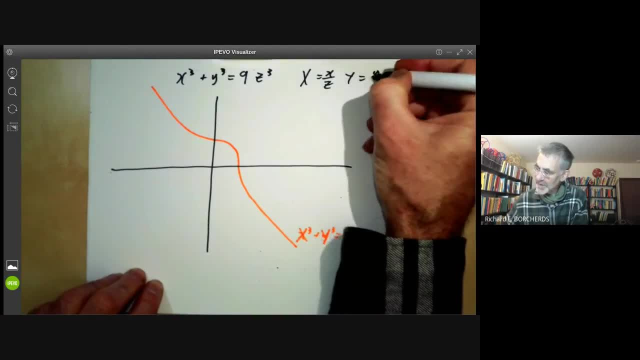 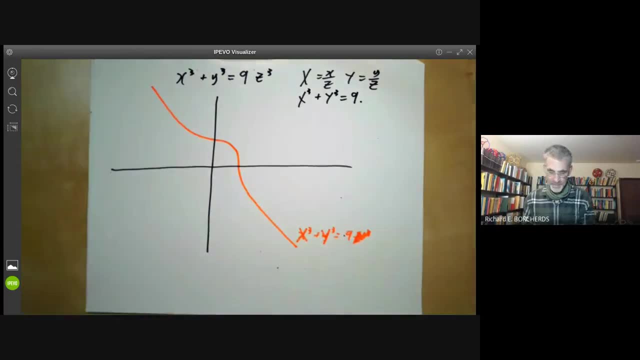 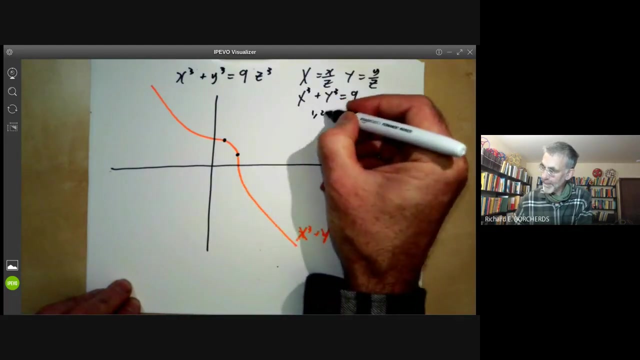 So let's put x equals x over z and y equals y over z, And then we find x cubed plus y cubed equals nine. And we know two points on this, because we've got the point one two and the point two one. 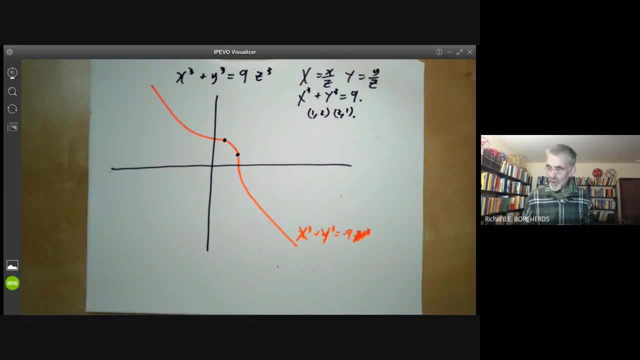 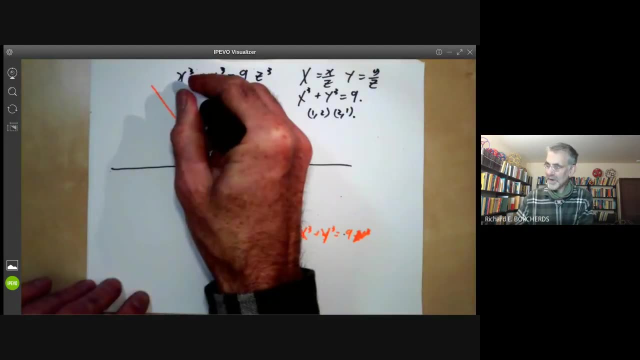 And how can we find other points on this? Well, one idea is we could just draw a straight line through these two points, but that wouldn't be very interesting because the straight line would just go like that and it would intersect this orange curve at infinity. 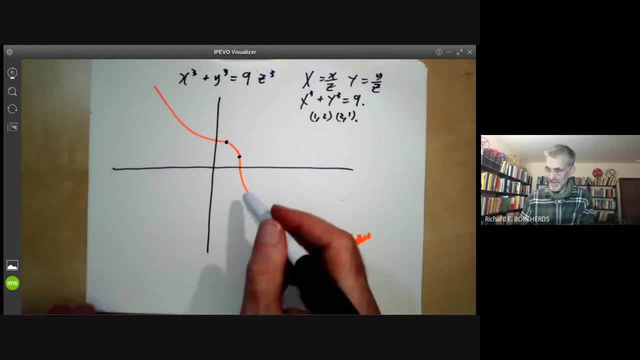 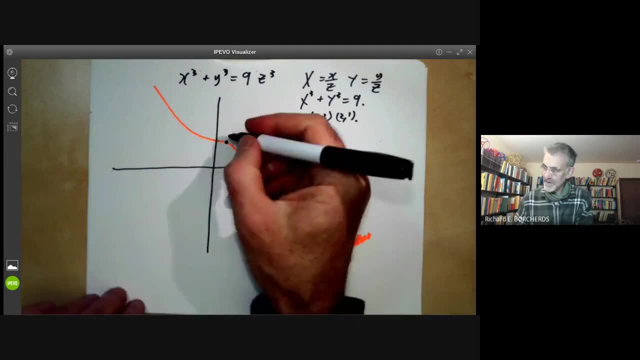 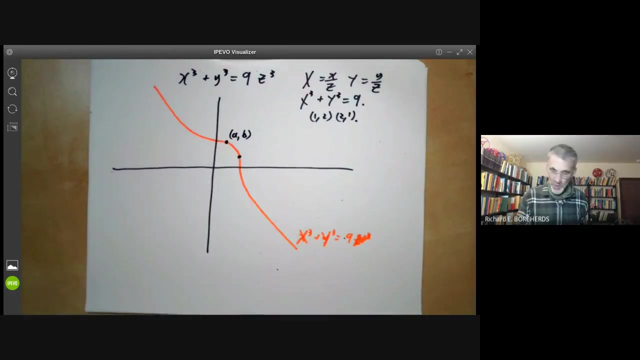 but it wouldn't have a third intersection point with finite coordinates. So what else can we do? Well, if we've got a point on this curve, let's call its coordinates a- b. for the moment, What we can do is we can draw the tangent. 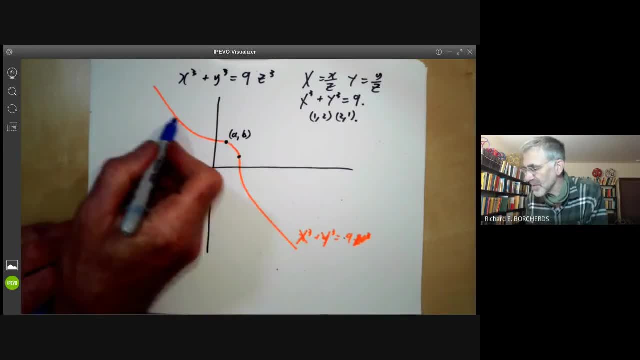 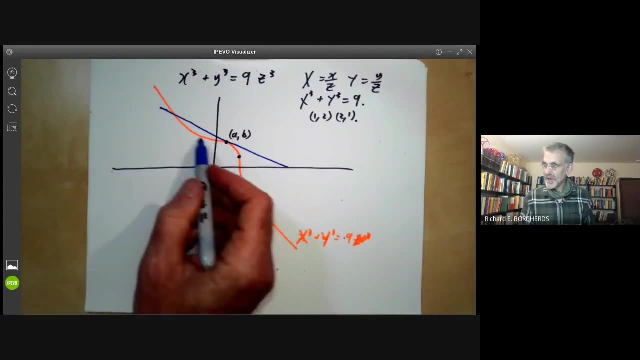 to the orange curve at this point. So it looks something like this: So here we've got a straight line and it intersects this orange curve in three points and it sort of intersects it twice at this point here because it's a tangent vector. You see, a tangent vector sort of intersects a curve. 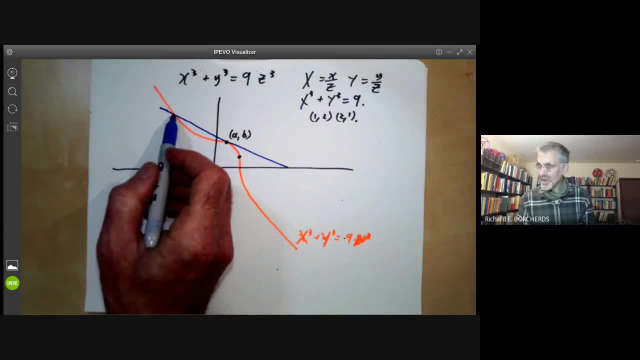 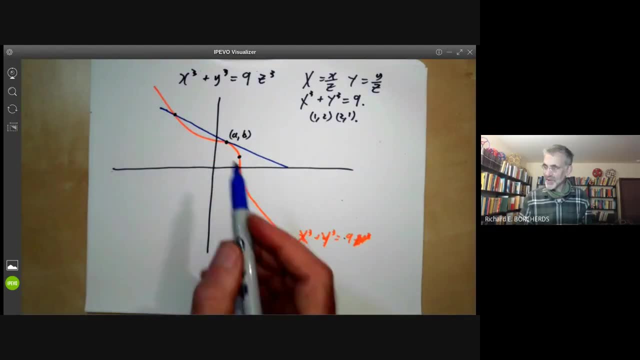 twice at one point. So as usual, this means the third point of intersection will also have rational coordinates. So we've got this very simple geometric idea. If we take a tangent vector to a solution and find the third point of intersection, it will give us another solution. 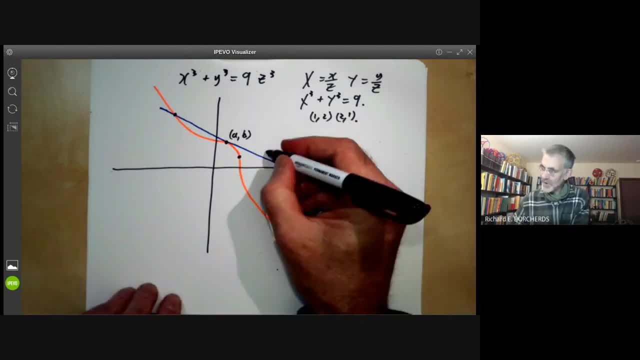 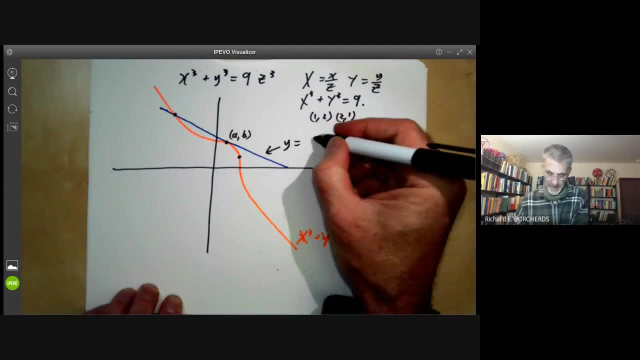 So let's do this. First of all, we need to work out the coordinates of the tangent line. Well, we work out the slope of the tangent line, which is minus a squared over b squared, And then we can complete the tangent line. 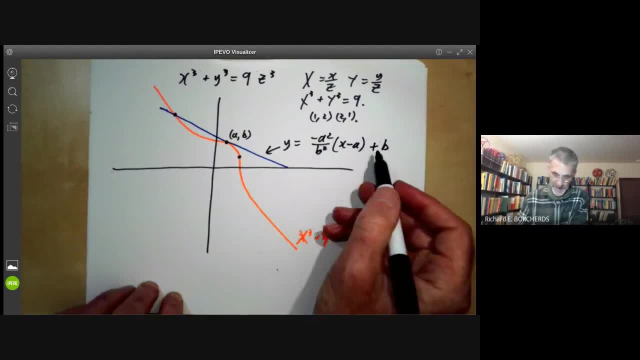 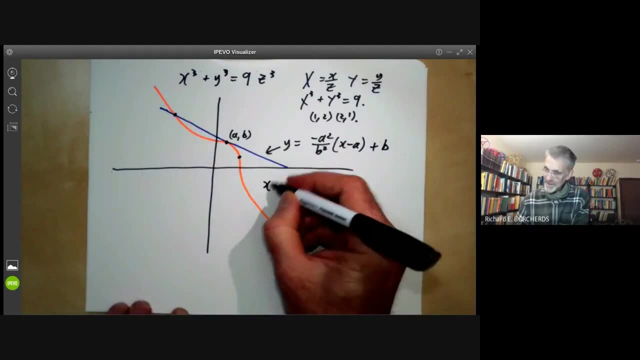 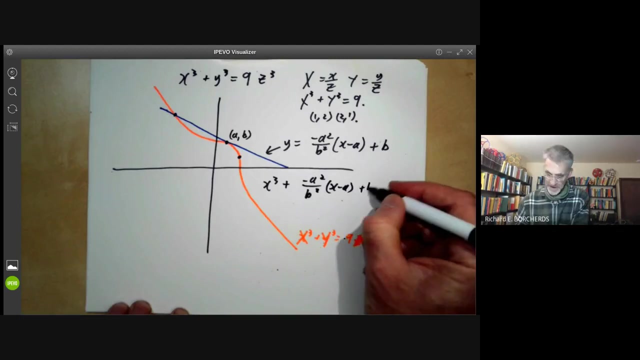 as x minus a plus b. So it's beginning to look a bit messy. And if we substitute this into this equation here we find we get x cubed plus minus a squared over b squared x minus a plus b, all cubed equals nothing. 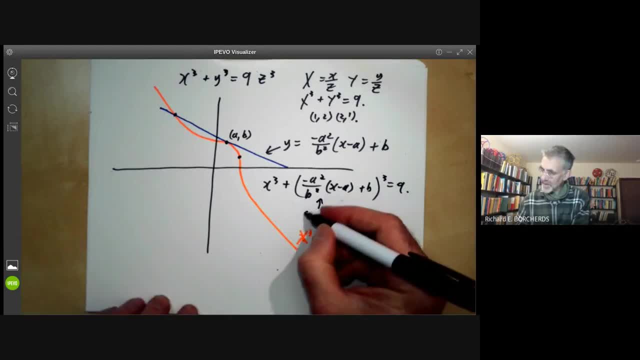 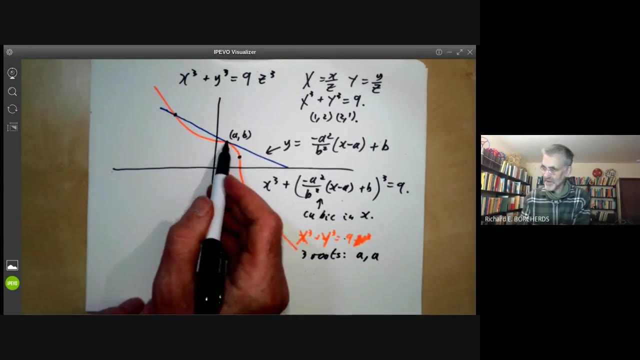 And the tangent vector is going to be the tangent vector of the tangent line And this is a cubic in x And it's got three roots. So two of the roots are a, because it intersects this orange curve twice at a and there must be a third root. 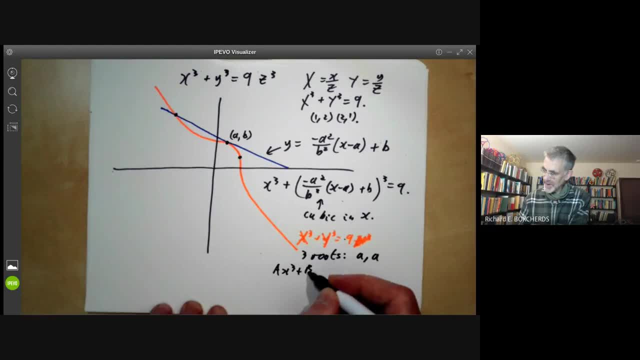 Well, if you've got a cubic equation: bx squared plus cx plus d equals 0, you know the product of the roots is going to be minus d over a. So we can work out the third root just by saying the product of a and a in the third root. 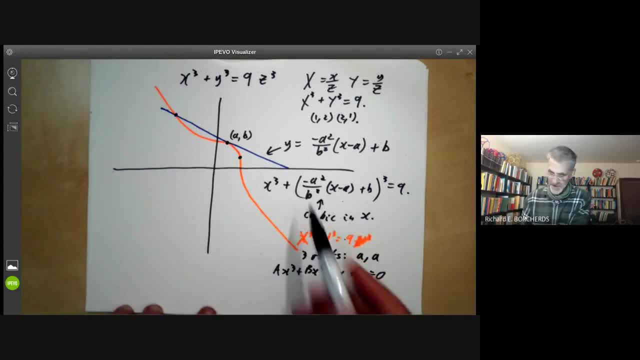 is minus the constant term of this, divided by the coefficient of x cubed, And if you work this out, it turns out to be minus a cubed plus b cubed, all cubed plus 9b to the 6th, divided by b to the 6th. 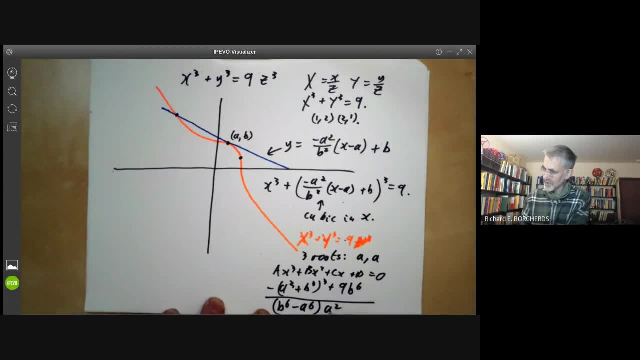 minus a to the 6th, And then we have to divide by the two roots we thought of. You can simplify this a bit, because we know a cubed plus b cubed is equal to 9,, for example. But anyway, so we have an explicit formula for the third root, x. 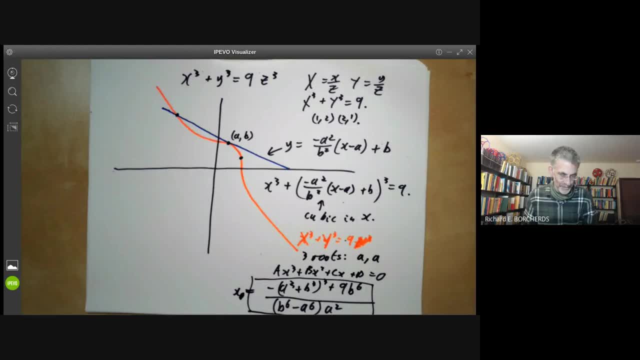 x is now equal to this, And similarly you can find y, So, for example. so if we found one root, we can now find another, So let's take ab to be the root. we already know about 1, 2.. Well, 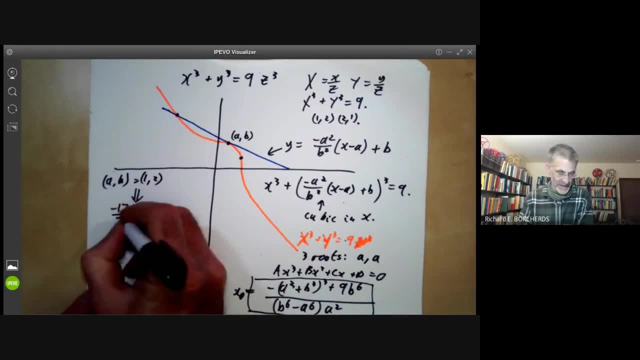 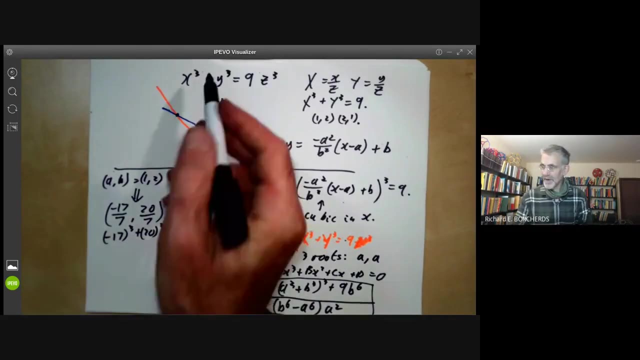 this gives us the root: minus 17 over 7, 20 over 7.. So we find: minus 17 cubed plus 20 cubed equals 9 times 7.. So we found another solution of this. Well, there's another way of finding solutions. What we 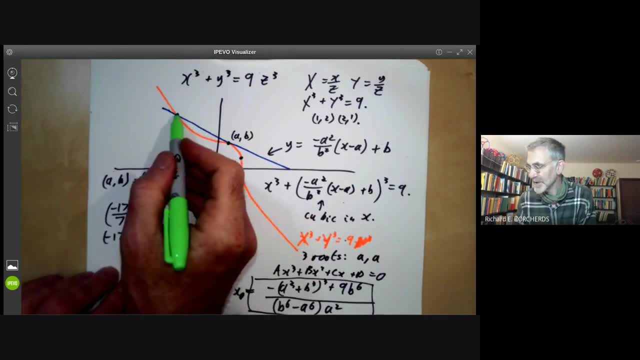 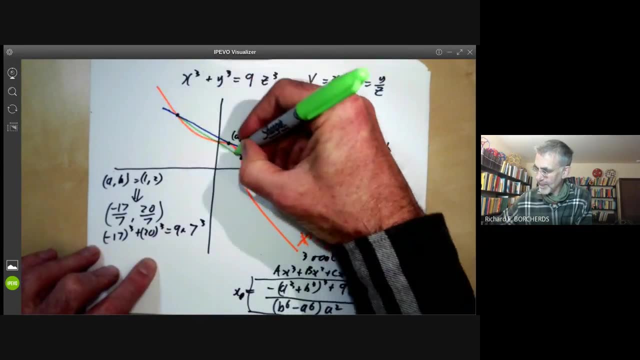 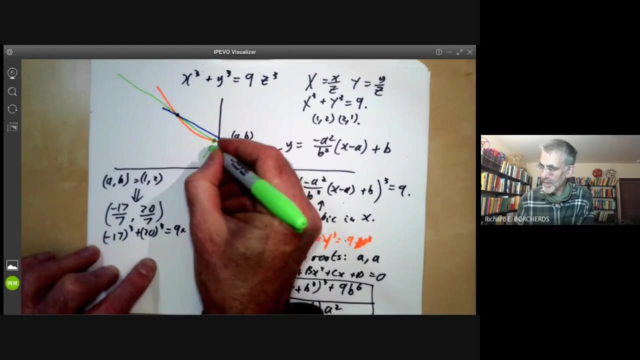 could do instead of taking a tangent line, is we can take any two solutions, say this one and this one, and draw the line through these. So this will intersect in a third point And, just as before, if these two solutions are the same, then we can take any two solutions and draw the line through. 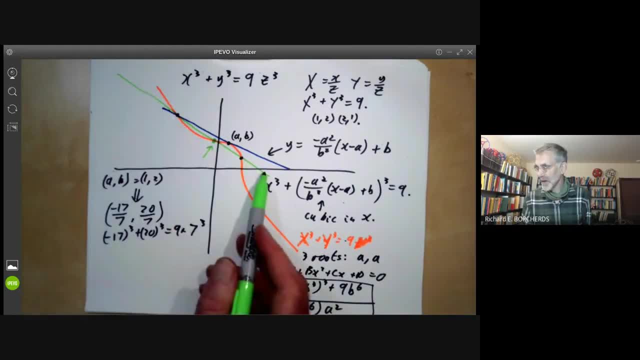 So this will intersect in a third point. And, just as before, if these two solutions are the same, then we can take any two solutions and draw the line through these. So this will intersect in a third point. So these two points are rational. The coefficients of this green line will be rational, So its 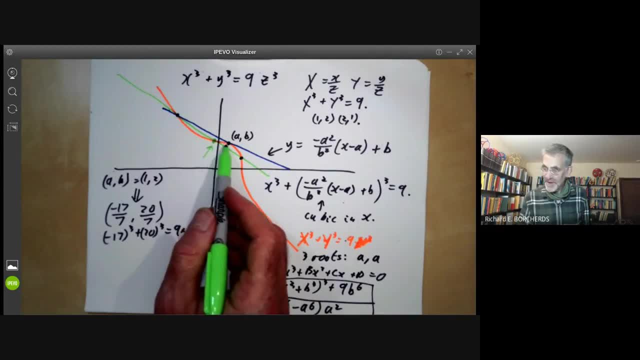 intersection with the orange curve will again have rational coordinates. If you do this, the algebra becomes really a bit of a mess. So I'm not actually going to carry it out explicitly, But I'll just give an example. So if you take this point and this point 2,, 1,. 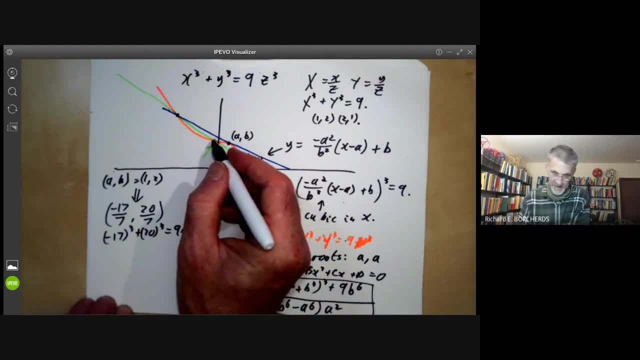 and draw the tangent line through them and work out its intersection point. it turns out to be minus 2, 7, 1 over 4, 3, 8, 9, 1, 9 over 4, 3, 8.. 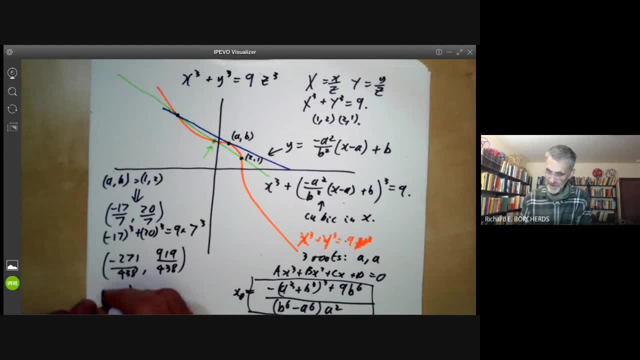 And this gives us the solution: minus 2, 7, 1 cubed plus 9, 1, 9 cubed equals 9 times 4, 3, 8 cubed, which, as you see, would be a bit tiresome to find by trial. 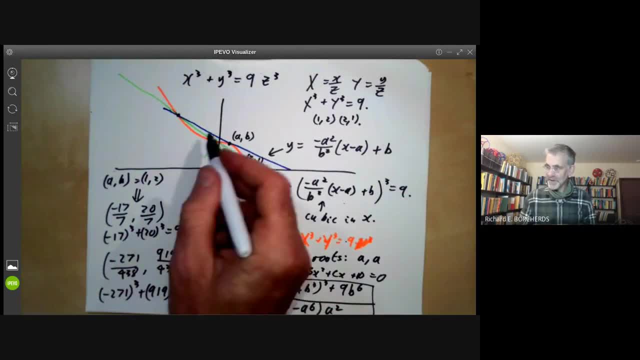 And using this geometric argument, it's quite easy to find solutions like this, And obviously you can just keep on doing this as long as your patient holds out. Every time you find a point, you can take tangent line. Every time you find two points, you can draw a line through them. 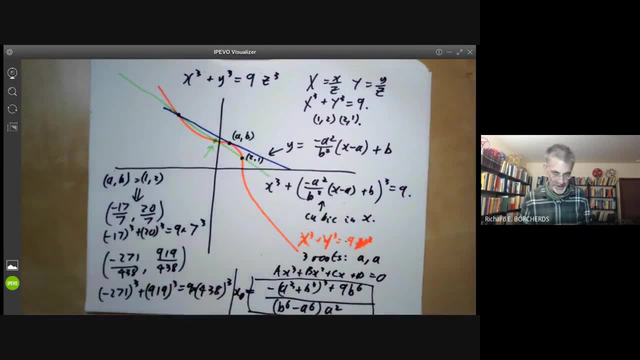 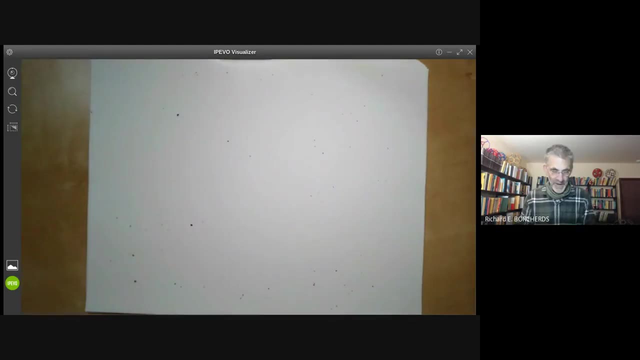 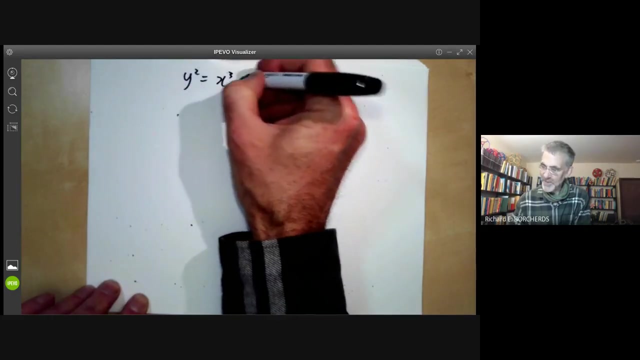 So you can generate endless numbers of integer solutions to this equation in a fairly systematic way. So the there's actually a famous theorem related to this due to Mordell which says: suppose you take any reasonable cubic equation, So for instance, y equals x. cubed minus x might look something like this: 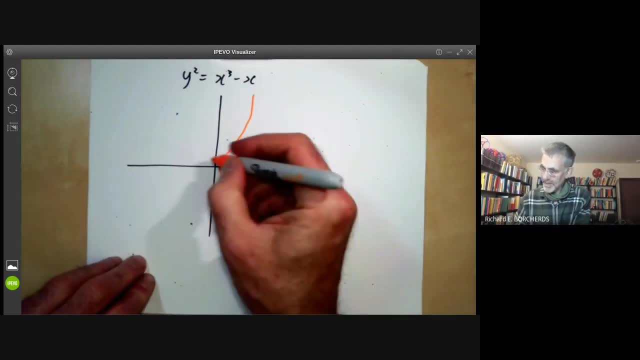 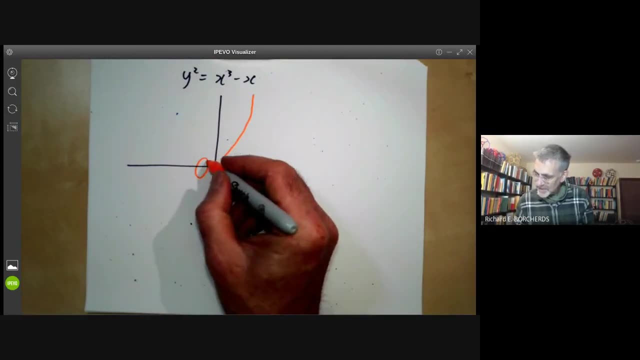 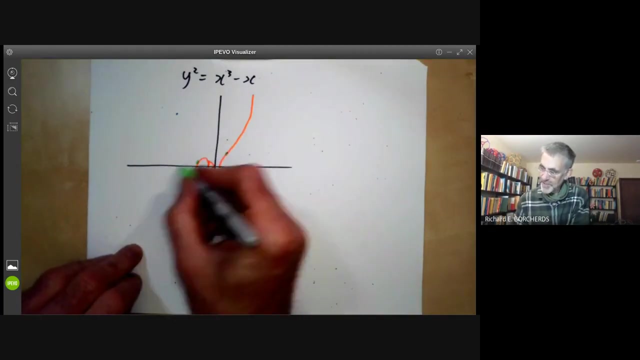 What you can do is: I guess it should go through the origin. never mind, you have to pretend, Yeah. What you can do is: whenever you've got three points on this, on this cubic, whenever you've got two points. 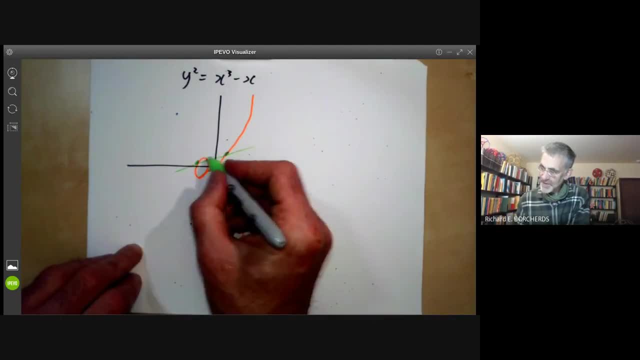 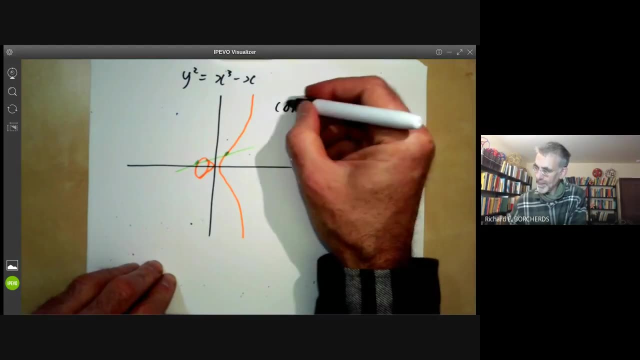 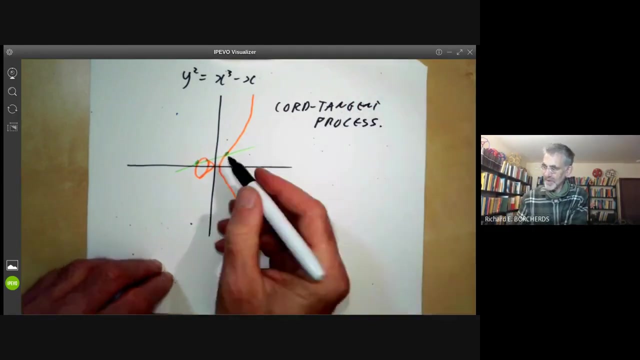 you can generate a third point by drawing a line through your first two points. This is called the chord tangent process, Or finding solutions, because you can either draw a tangent to a point you found or you can draw a chord through two points. 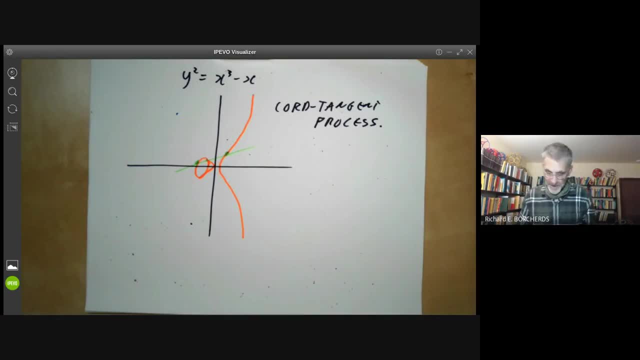 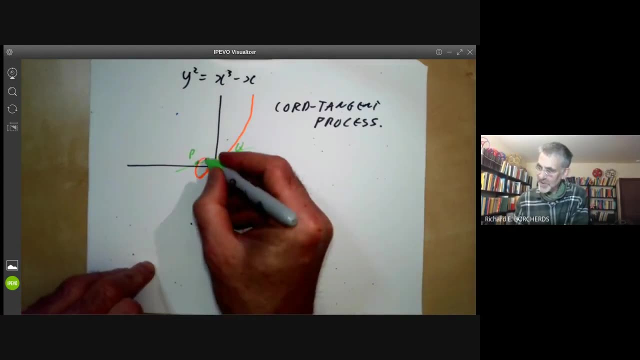 And it turns out that you actually get something called a group. So suppose I've got two points, P and Q, here. Then I get a third point here, and if I change its y coordinate to minus the y coordinate, I get another point that I'm going to call p, sort of plus q. 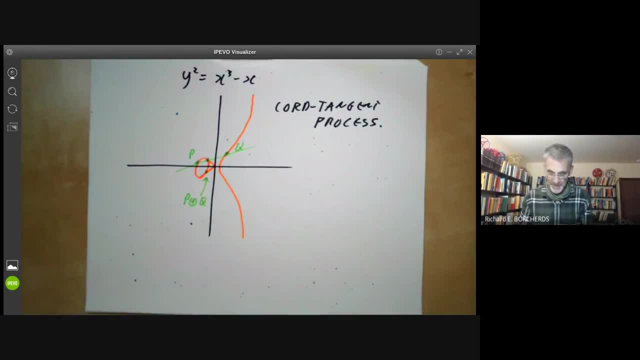 It's a funny sort of addition And it turns out that this funny addition of points behaves obeys the usual rules of algebra. So p plus q, q is obviously equal to q plus p, because the line through p and q is the same as the line through q. 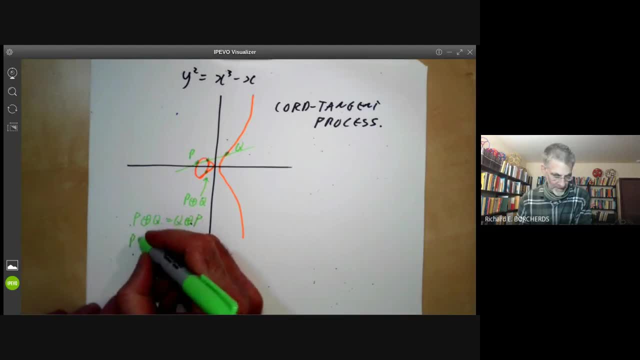 and p A slightly more difficult fact is that p plus q plus r is equal to p plus q plus r. This is really a total mess to verify because the formula for the coordinates of p plus q are really rather complicated and trying to calculate this explicitly is really rather a headache. 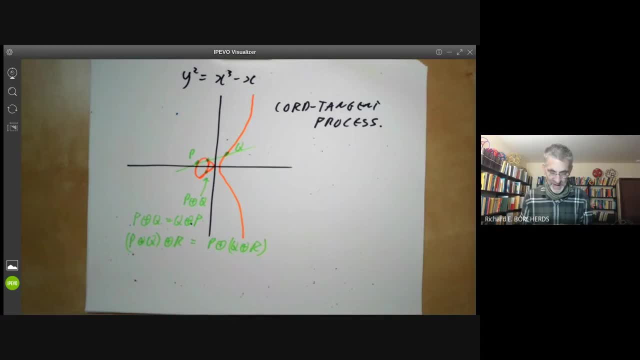 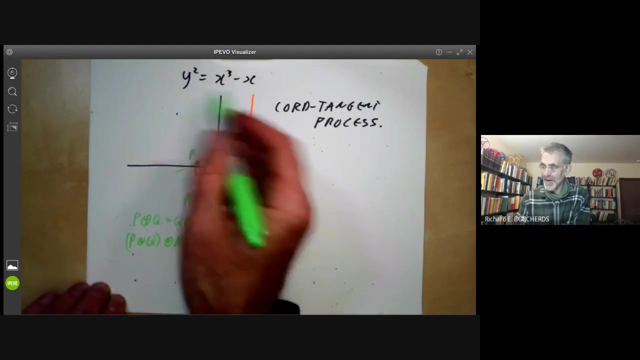 There is actually an easier way to prove this without doing explicit calculations, but whatever. So what we get is a sort of funny addition of points which obeys the usual rules of algebra, and Poncurri asked this question: can you find a finite number of rational points on any cubic? 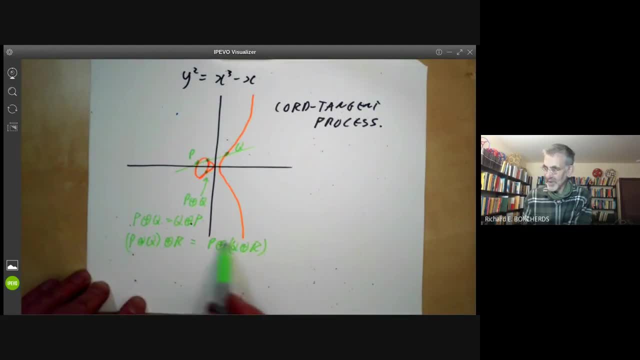 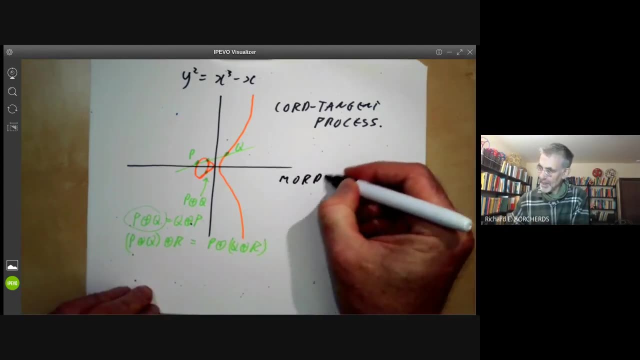 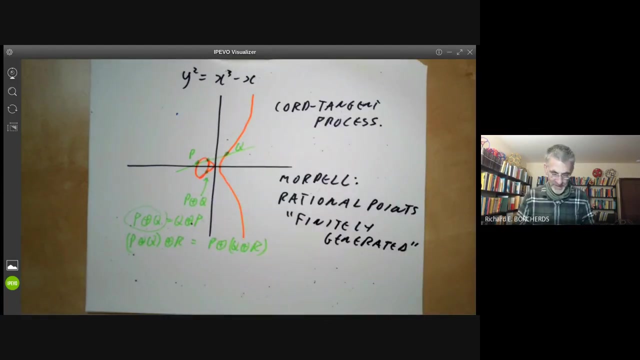 so that all rational points can be obtained from this finite number by using this operation? And Mordell showed. the answer is yes. He showed the rational points are finitely generated. In other words, you can find a finite number of rational points such that all the other rational points are generated from these by the chord tangent process. 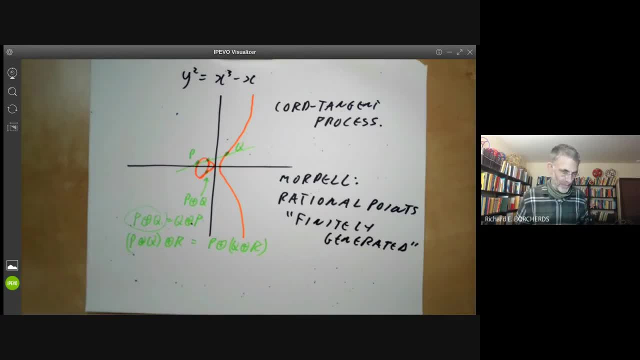 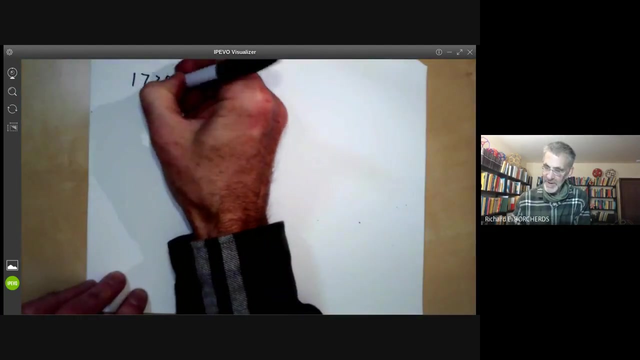 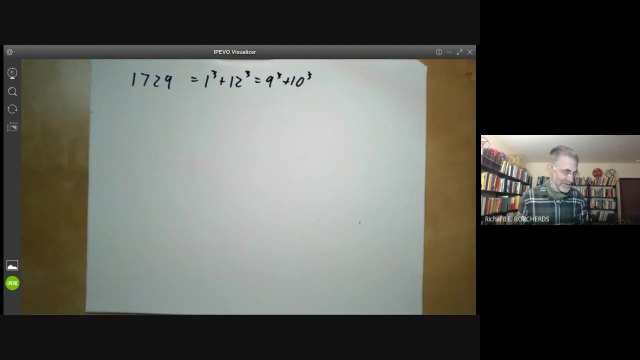 So that's it. So now we're. so far we've been looking at curves. now I'm going to look at an example of a surface. So this is related to Ramanujan's famous number. So there's a famous mathematical anecdote about this and this appears in Hardy's book on 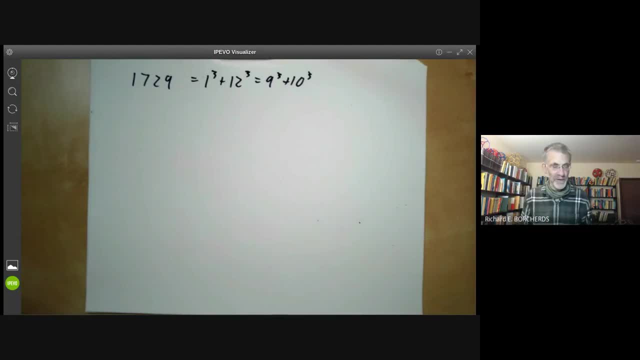 Ramanujan. so I have here a copy of Hardy's book. Hardy's book, And on page 12, he has this anecdote that I'll just read out. So Hardy says: I remember going to see him once when he was lying ill in Putney. So he's talking about. 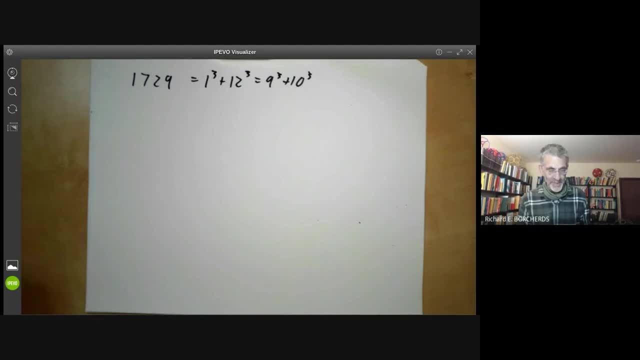 remanagement. of course I had ridden in taxi cab number 1729 and remarked that the number seemed to me a rather dull one and that I hoped it was not an unfavorable omen. No, he replied, it is a very interesting number. It is the smallest number expressible as the sum of two. 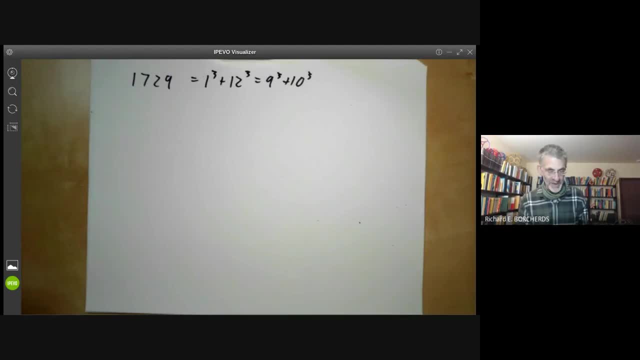 cubes in two different ways. I asked him, naturally, whether he would tell me the solution of the corresponding problem for fourth powers, And he replied after a moment's thought that he knew no obvious examples and supposed the first such number must be very large. So, as a result of 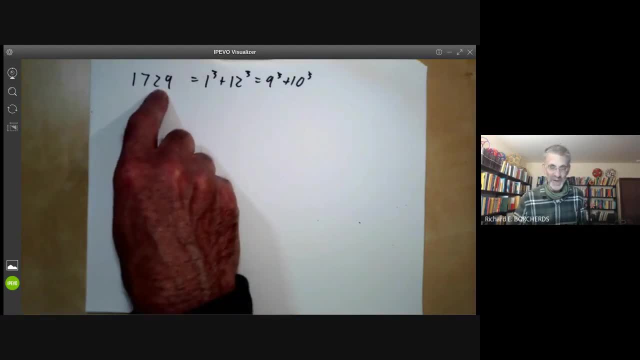 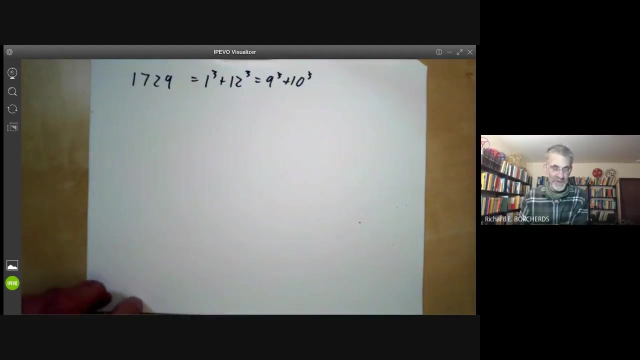 this story, this particular number, 1729, has become really famous. It's even got its own Wikipedia article, if you want to read about it. So what I'm going to do is show how to find other examples of numbers with this property. So we want 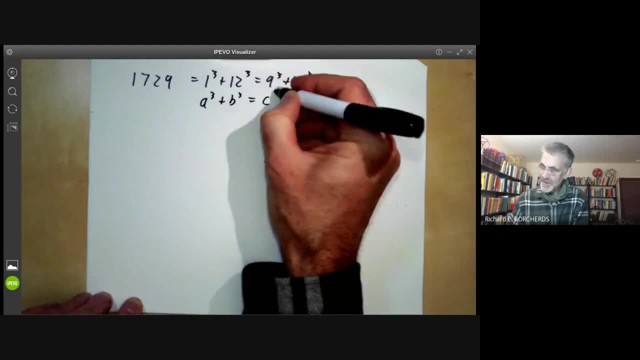 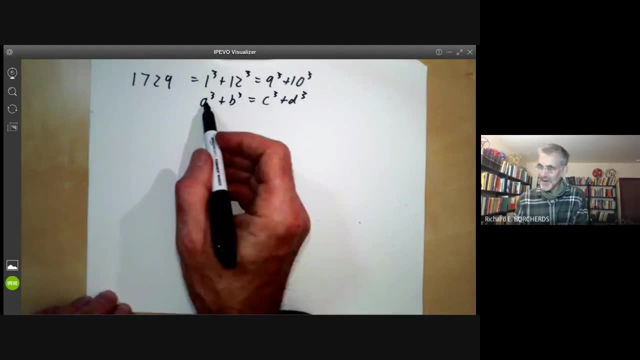 to solve: a cubed plus b cubed equals c cubed plus d cubed. And obviously we want non-trivial solutions where a isn't equal to c or d and it's not equal to minus b, and so on. You can rearrange. 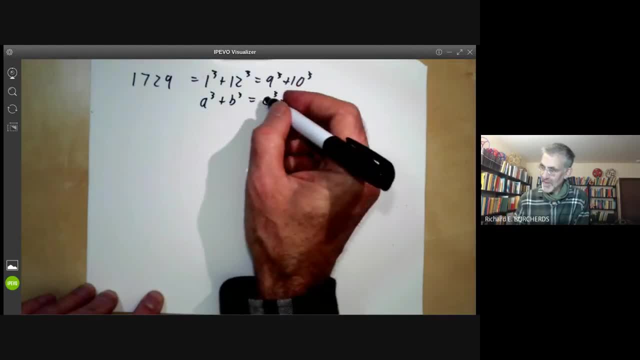 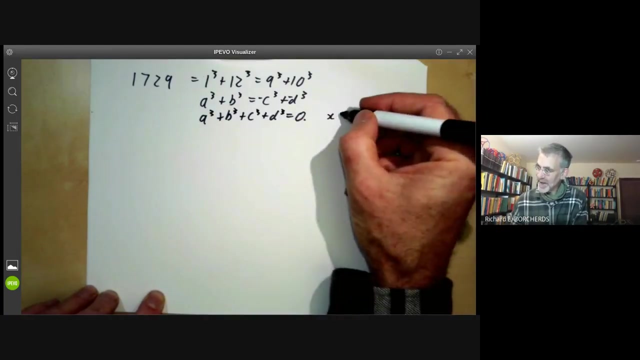 this by changing the sign of c and d. So we get a small�를 function of d cube, so it becomes a bit more symmetrical. So it looks like that, And now we can just divide by d cubed. So let's put x equals. 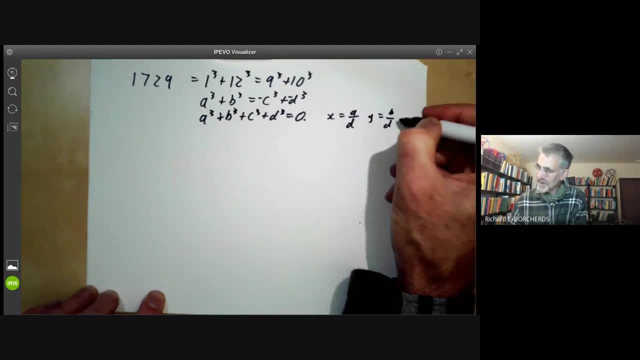 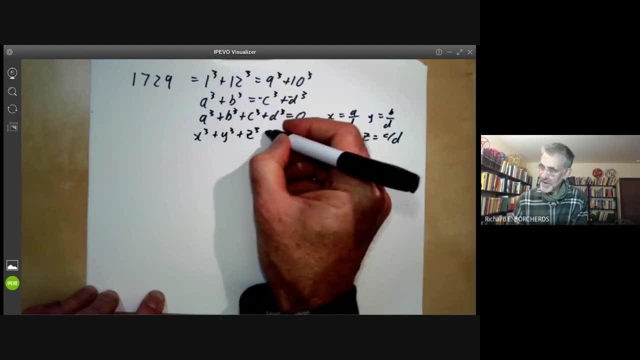 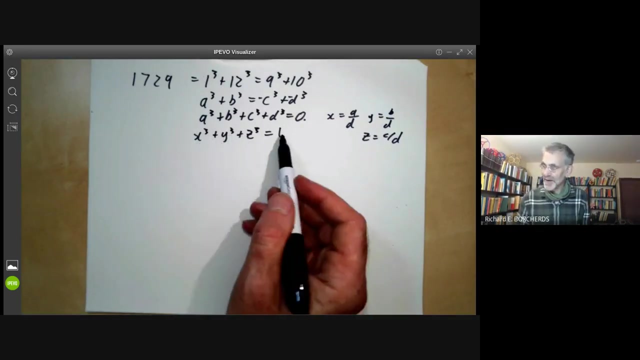 a over d, y equals b over d, z equals c over d. So we get x cubed plus y cubed plus c cubed, equals 1.. So this is a bit like the earlier equation. We had x cubed plus y cubed equals 9, except. now we've got c down the herself, So there's there's some Elvinism to that. It a problem, hem, Therefore smooth bigger times in n, But that's fine all year round. So just nice to be smooth, bigger, nice to be together. The other strong point found here is that that's also an enumeration. 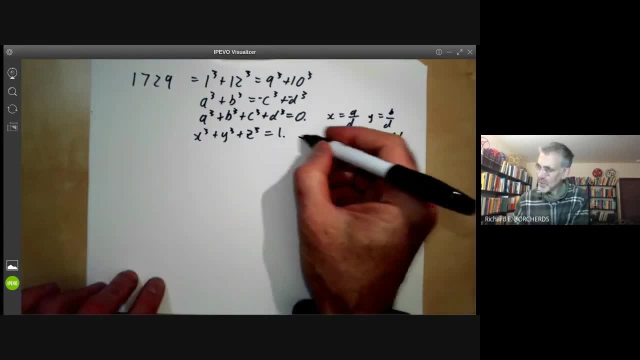 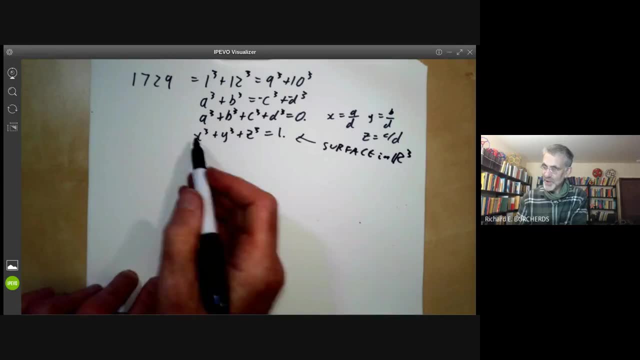 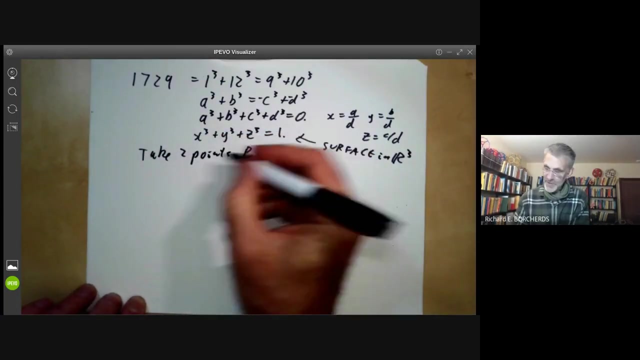 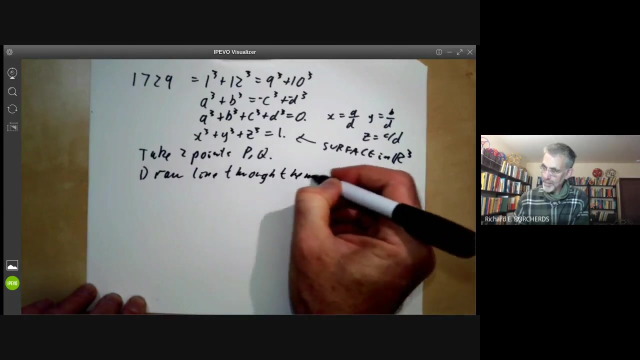 we've got three variables and this is now the equation of a surface in real three-dimensional space, and we're trying to find points on this surface with rational coordinates. And now we can do a similar trick that we did with cubic curves. Let's take two points, P and Q, and draw a line through them and this line. 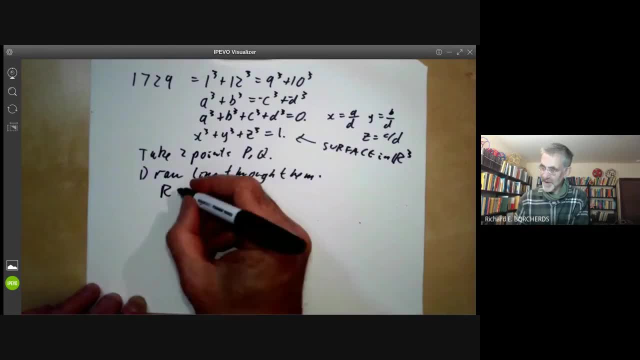 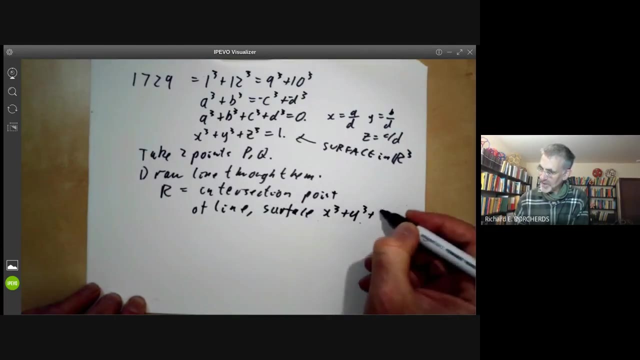 will usually intersect this cubic surface in another point. so R is the intersection point of this line and the surface X cubed plus Y cubed plus C cubed equals one, assuming it line intersects this Occasionally the line would just be asymptotic to it. but we'll ignore that. 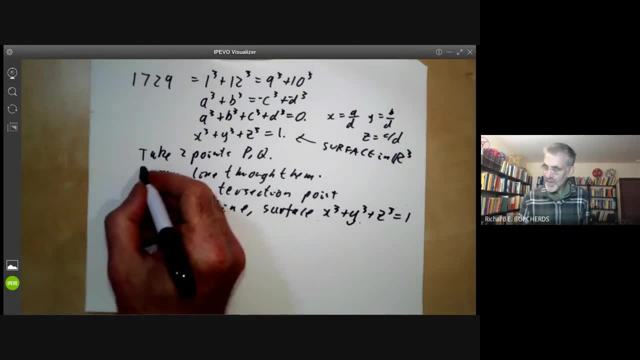 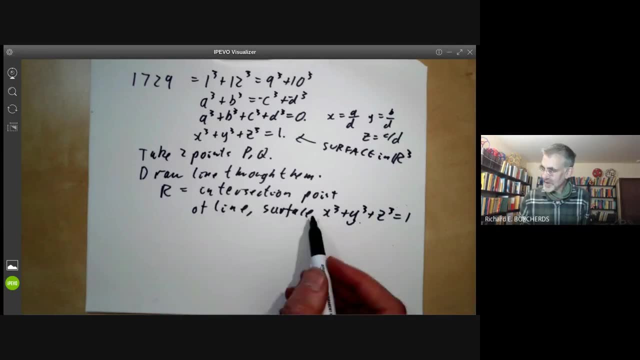 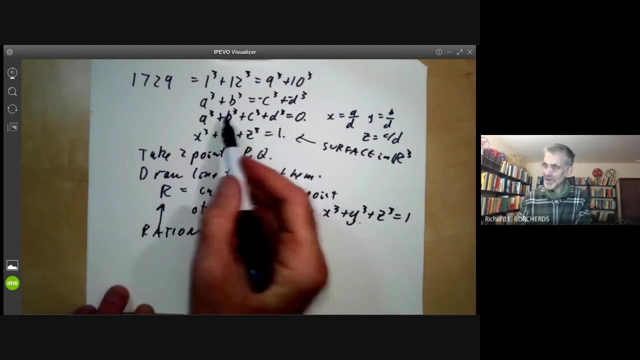 problem. And now, just as before, if P and Q have rational coordinates, then the equation of this line will have rational coordinates. so the third intersection point with this surface will also have rational coordinates. So this will be a rational point. Okay, well, let's try this. First of all, we notice this equation has lots of 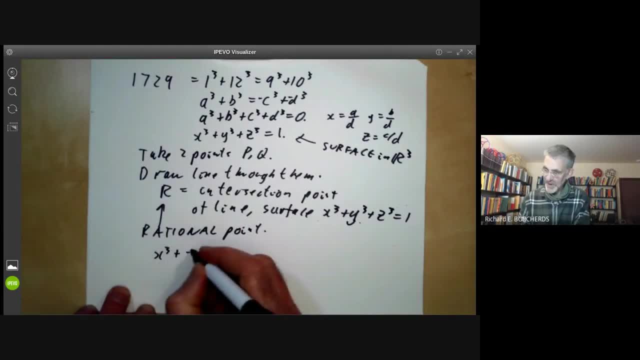 obvious solutions like it's got X cubed plus minus X cubed plus one cubed equals one cubed. and it's got Y cubed plus one cubed plus minus Y cubed equals one cubed. and one cubed plus C cubed plus minus C cubed equals one cubed. So these 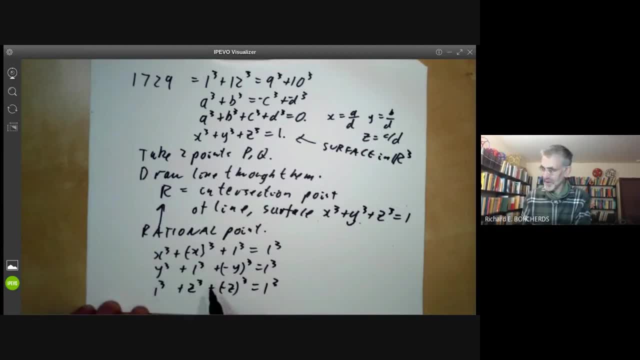 are the obvious, not very interesting solutions And we can ask what happens if we take two of these boring solutions and do this process. we draw the line through them and take the third intersection point and the answer is you get a third uninteresting solution. So if 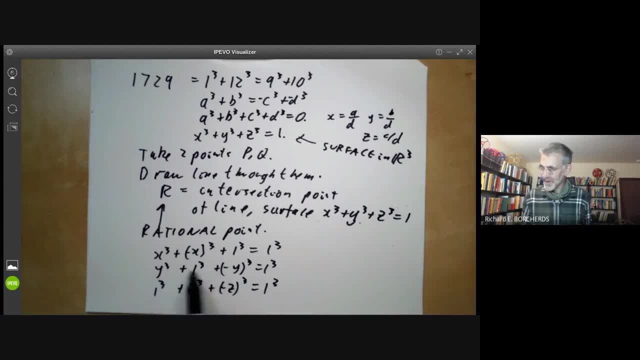 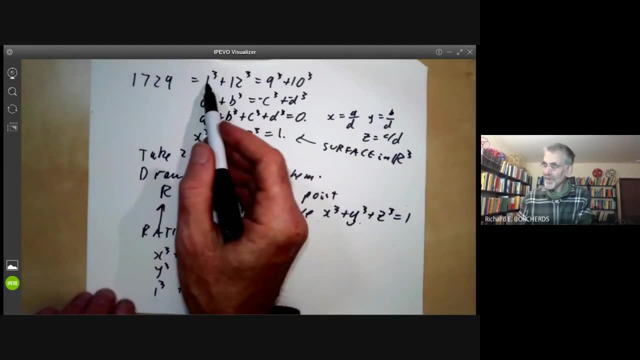 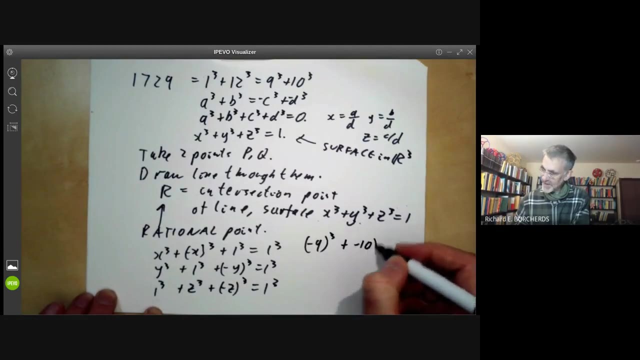 you take a point on with satisfying this and a point satisfying this and carry out this process. we just get a point here, So that's not terribly interesting. However, we've got a more interesting solution: minus nine cubed plus minus 10 cubed, plus twelve cubed plus one equals zero. so guess, 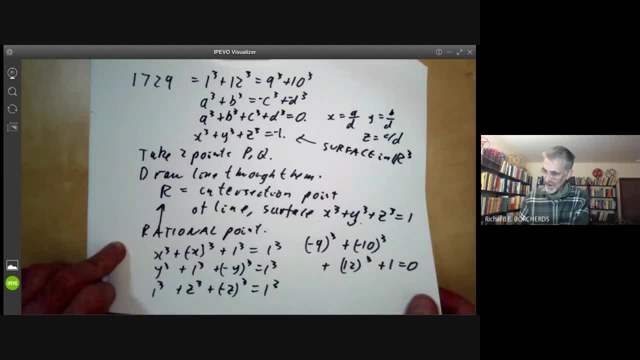 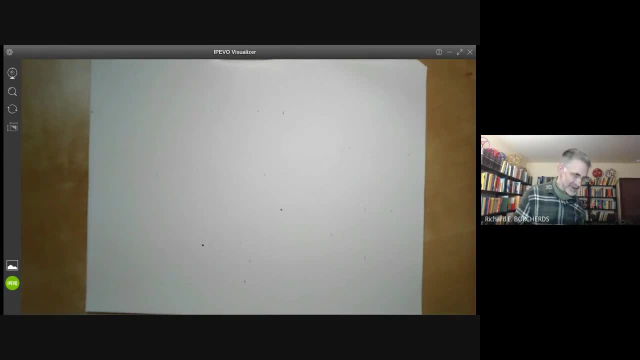 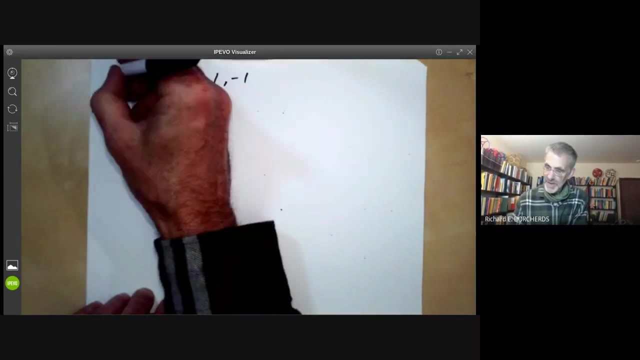 that should be a minus swan there, never mind, um. so what happens If we do this? well, let's just see. So let's take the point p to be 1 minus 1 minus 1, and we're going to let this be correspond to a. 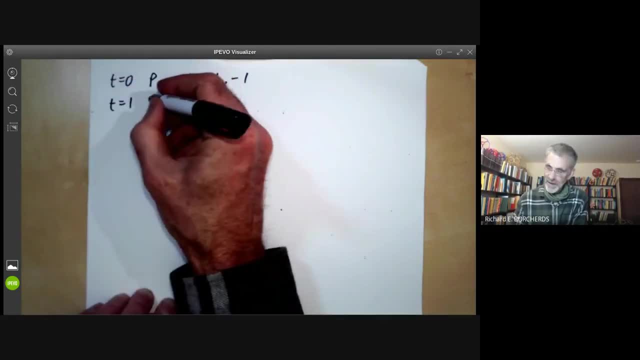 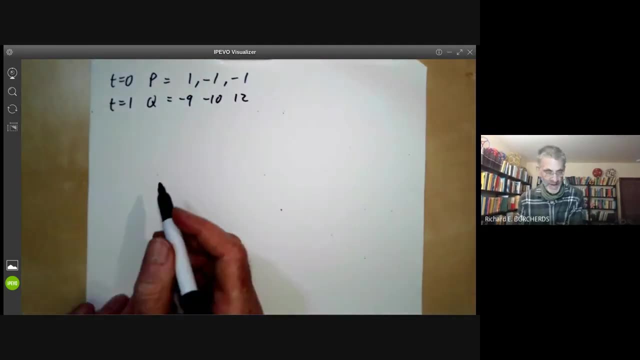 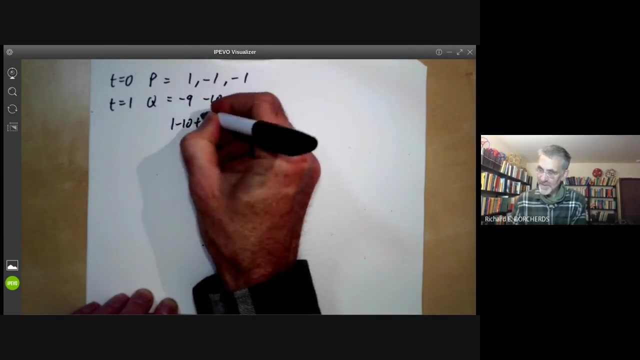 rational number t being 0, and at t equals 1, we're going to let it be the point Q, which is equal to minus 9 minus 10, 12, and now we're going to draw the line through these points and it will be the set of points 1 minus 10, t minus 1. 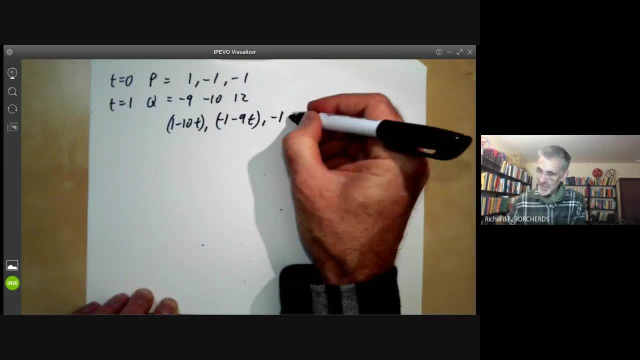 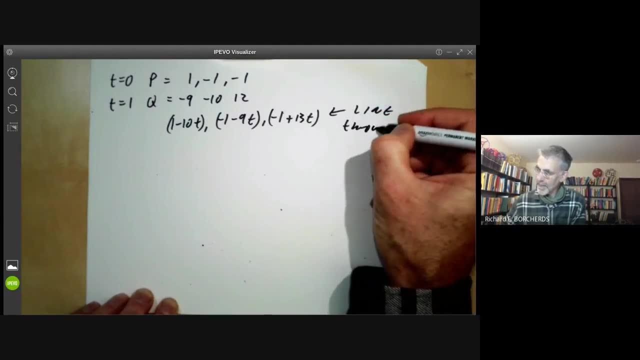 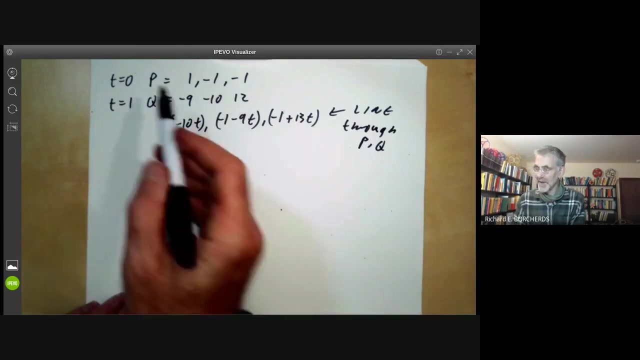 minus 9 t, minus 1 plus 13 t. so this is a line through P and Q, because you can see, it's a line parameterized by T and it goes through P and Q when T is 0 or 1. so this is going to be our third point, R, and now we want the sum of these three. 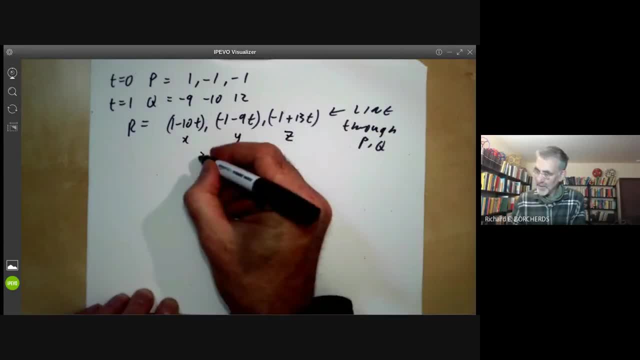 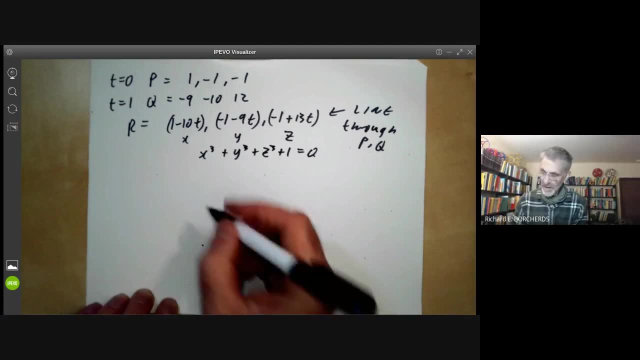 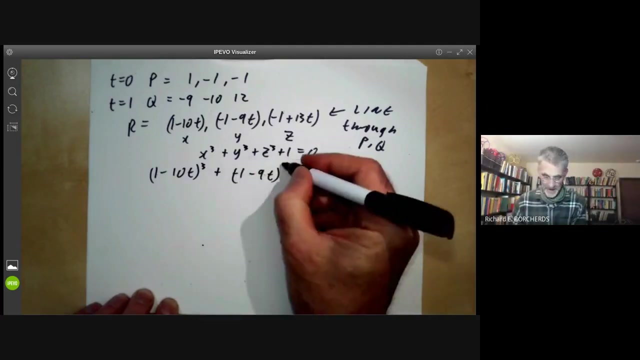 numbers cubed. you want x cubed plus y cubed plus c cubed plus 1 to be equal to 0. so we get 1 minus 10 t cubed plus minus 1 minus 9 t cubed plus minus 1 plus 13 t cubed. 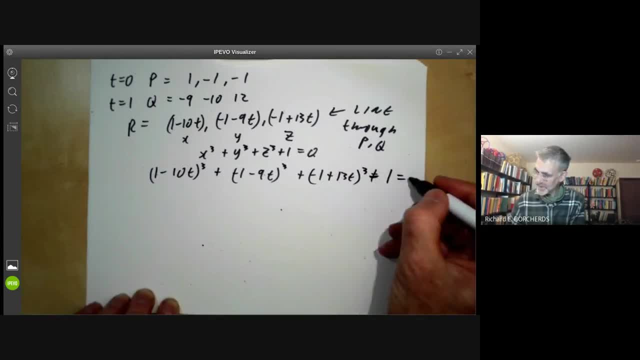 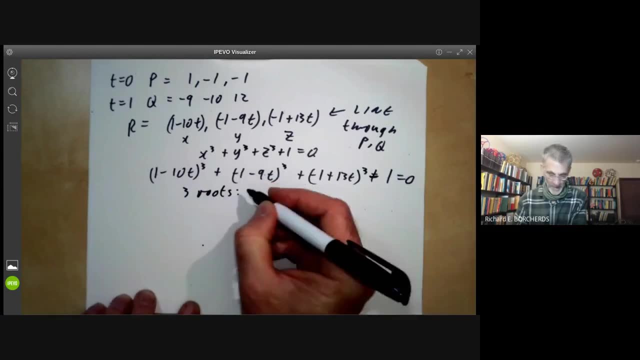 equals 1. so plus 1, 0. keep getting that the wrong way around and you can see that it has three roots. it is root t equal 0 or t equals 1, and the third root is going to be rational and you can work it out explicitly by doing some calculation. it turns out to: 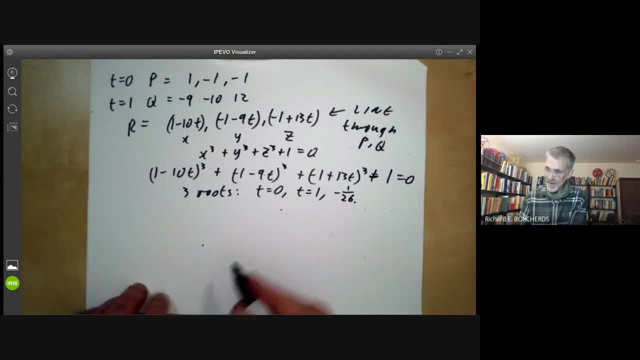 be minus 1 over 26 in this case. so we now find our point R is equal to 36 over 26 minus 17 over 26 minusan over 26.. so we get a solution there. that which is this: DSM is a 不是 norm. 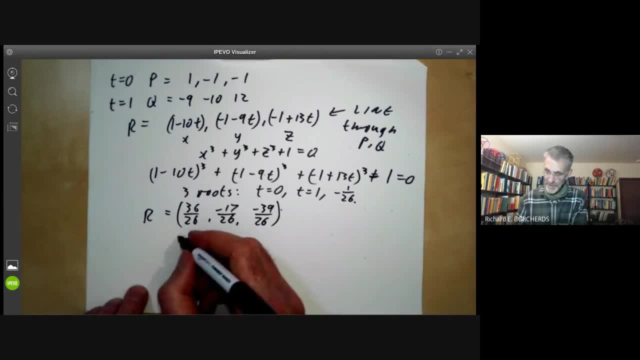 so we find a ك gates along the Radigny, Skysnun property and this셔. the 36 cubed plus 26 cubed equals 17 cubed plus 39 cubed. So we've got another solution to Ramanujan's equation. 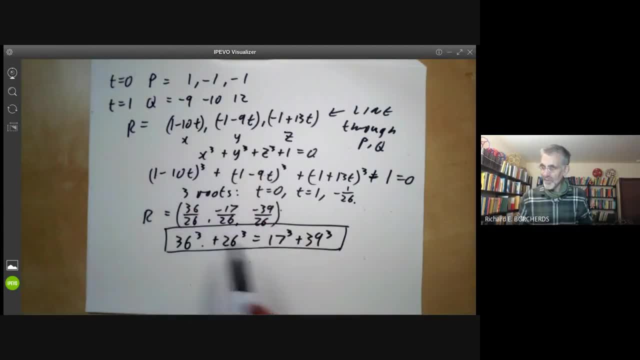 And obviously you can keep generating more and more solutions by just drawing a line through any two solutions you've got. And incidentally, you can ask if you get a group like this And the answer is you don't, because if the points P and Q are equal. 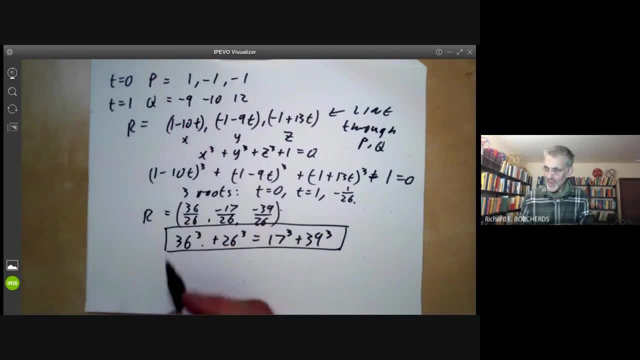 you think you would take the tangent line to P and Q. But the trouble is, if you've got a point of a surface, it doesn't have a tangent line. It has a tangent plane. So you don't really know which line tangent to it to take. 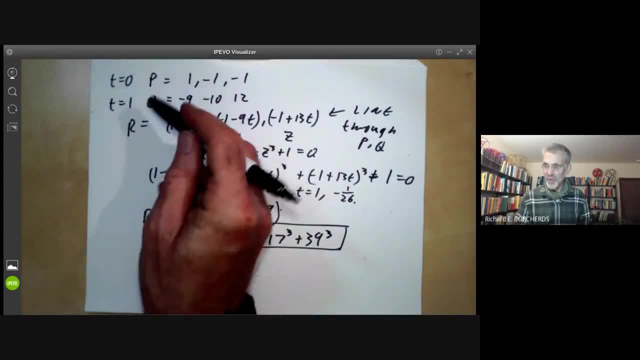 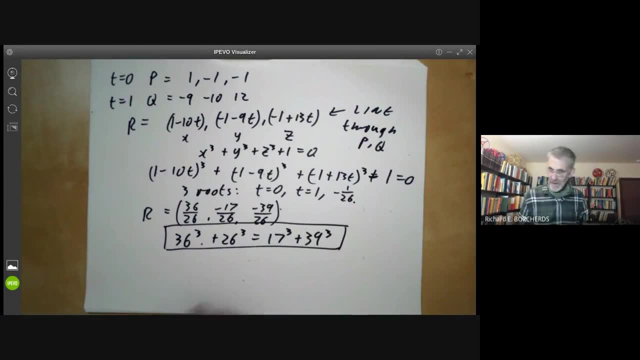 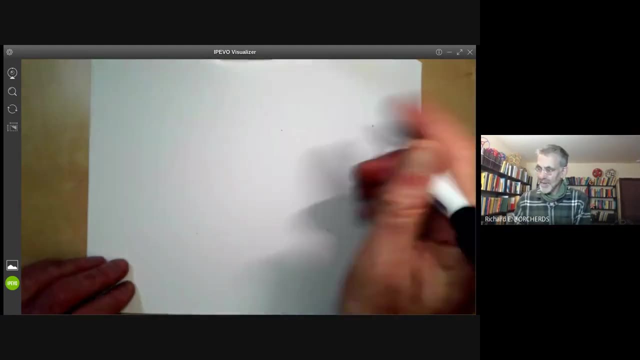 So you can't really define an addition operation on points because this breaks down if the two points are the same. So in general what happens for plane curves is if you've got a plane, if you've got a curve, then it might have degree two. 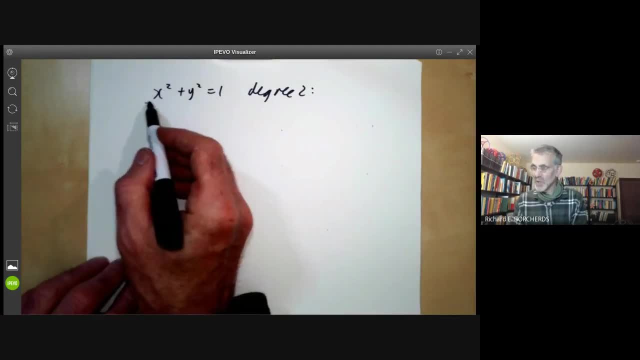 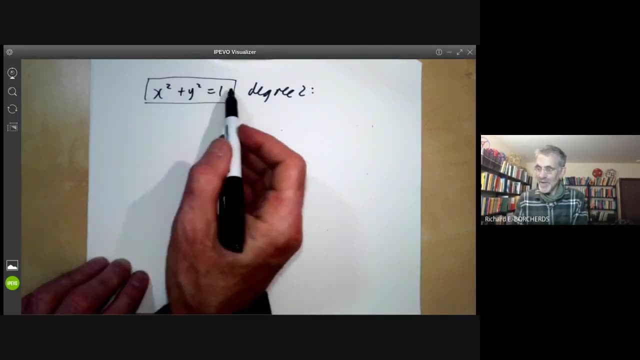 And if you've got a plane curve of degree two, it acts rather like the equation x squared plus y squared equals one. If we can find one rational point on it, then we can find all the other rational points Very easily just by drawing a line through both points. 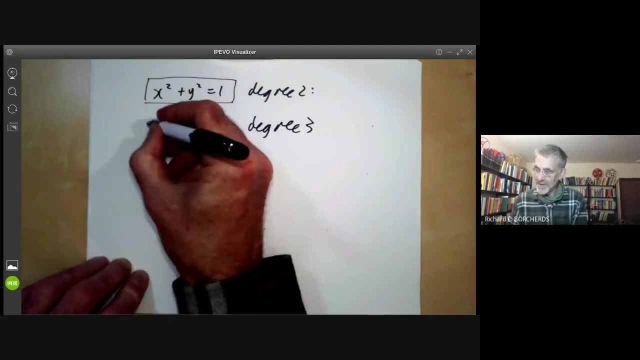 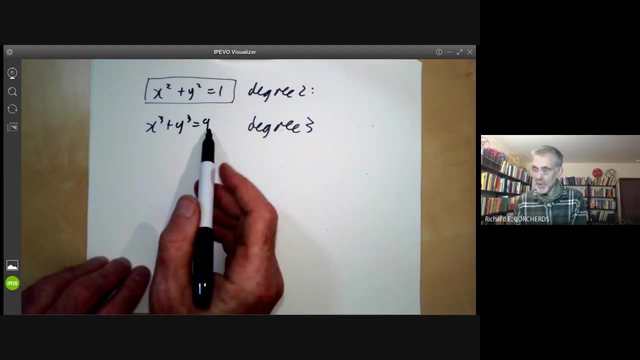 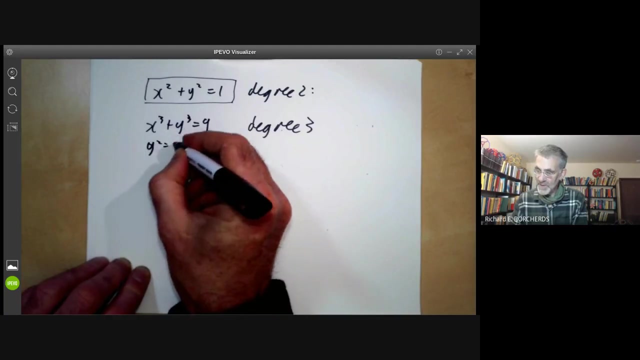 If we've got a degree three curve such as x cubed plus y cubed equals nine, then this is an example of something called an elliptic curve, unless it happens to be singular, such as the curve y squared equals x squared plus x cubed. 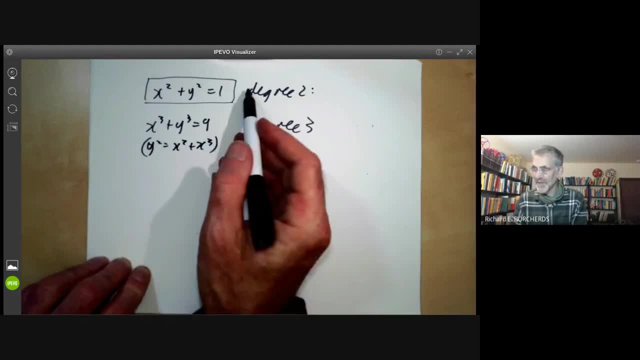 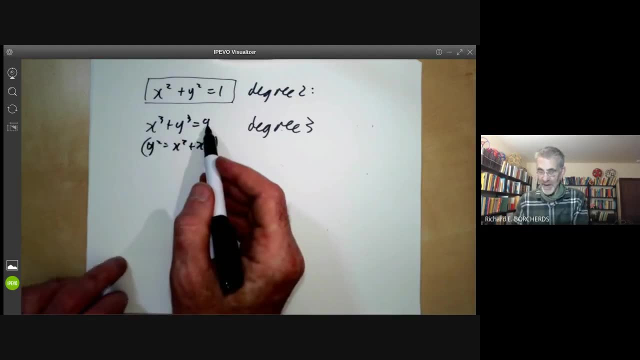 So singular elliptic curves with singularities behave a bit like degree two curves. Elliptic curves without singularities behave like the degree three curve we had. that Mordell showed you can find a finite number of points that generate all of them. What about curves of degree greater than three? 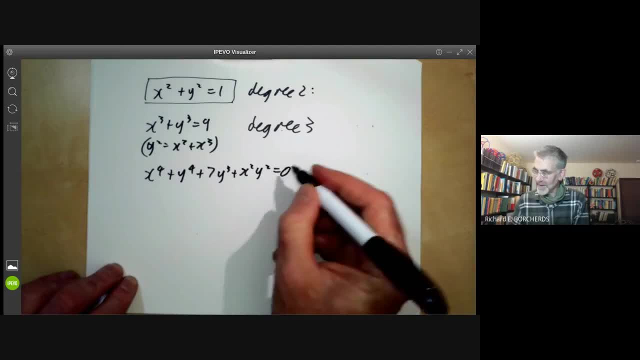 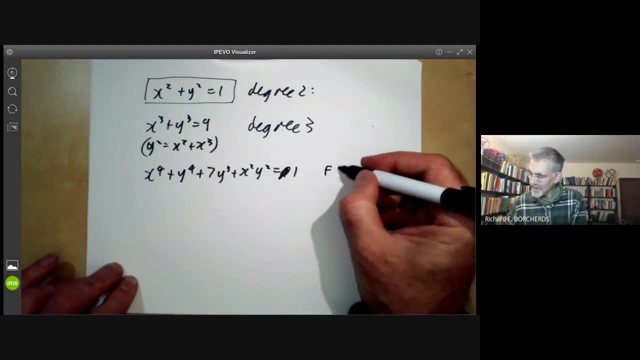 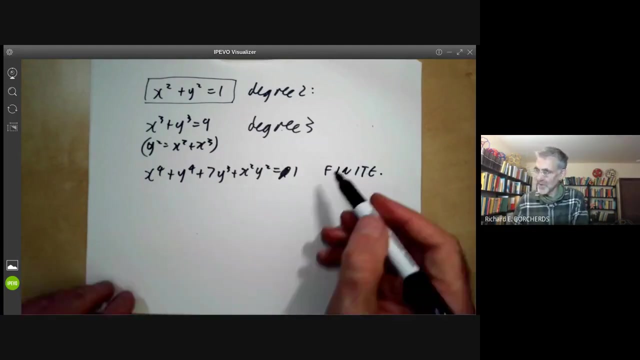 So if you have something like this, then curves of degree greater than three generally only have a finite number of rational points on them. This is a very deep theorem proved by Faulting's a few decades ago. It was originally conjectured by Mordell. 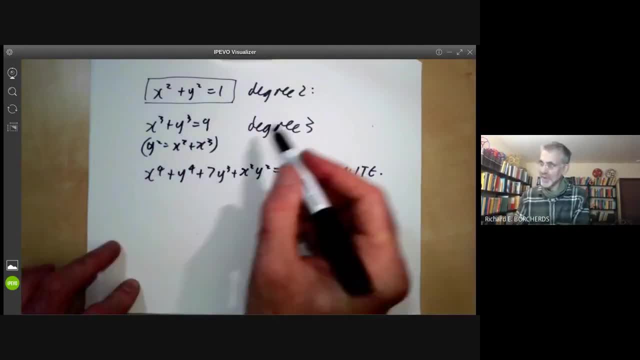 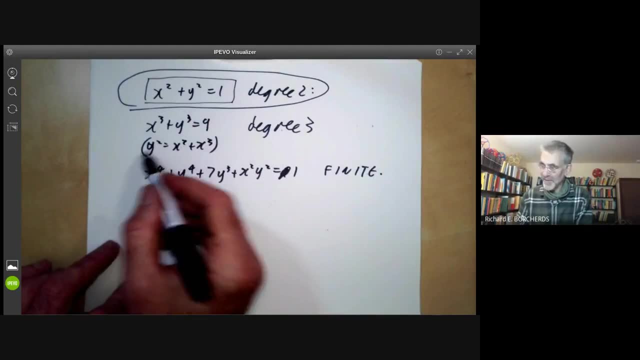 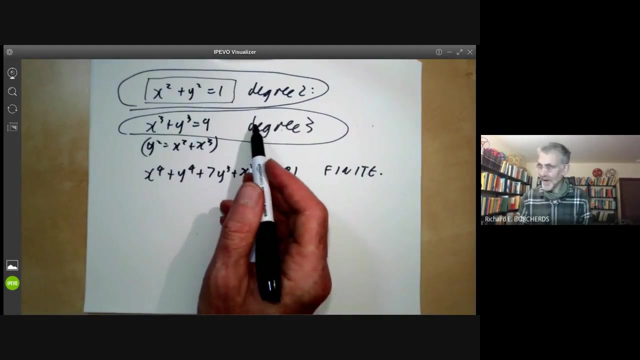 So, anyway, it turns out that curves split up into three different groups. There are those for which the rational points are really easy to find- an infinite number usually. Then we get elliptic curves, where the rational points are at least finitely generated. 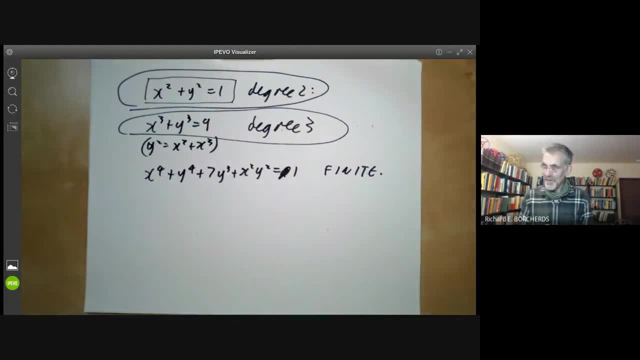 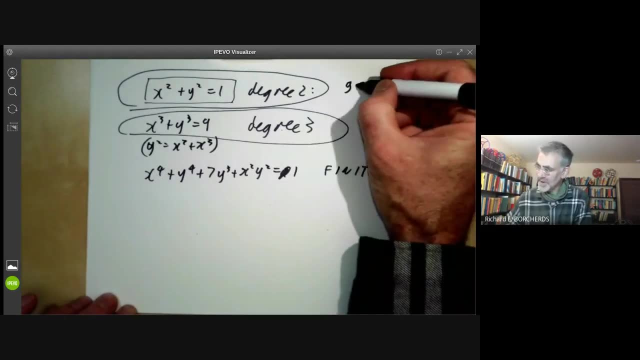 And then we get all the other curves where there are only a finite number of rational points and they seem to be very hard to find. These differ by something called the genus. We say these curves have genus zero, these curves have genus one. 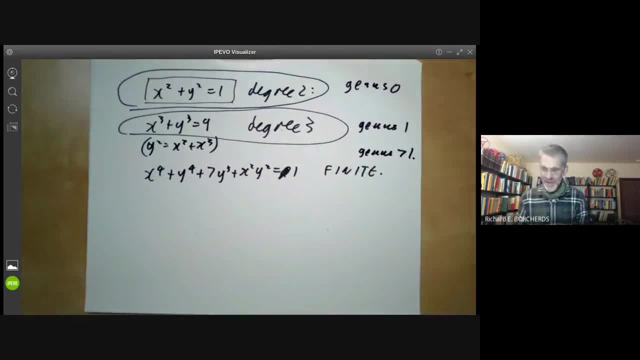 and these curves have genus greater than one, And the genus turns out to be what happens if you take the curve over the complex numbers, which gives you a surface, and then the surface has a number of sphere with a number of handles, and the number of handles is the genus. 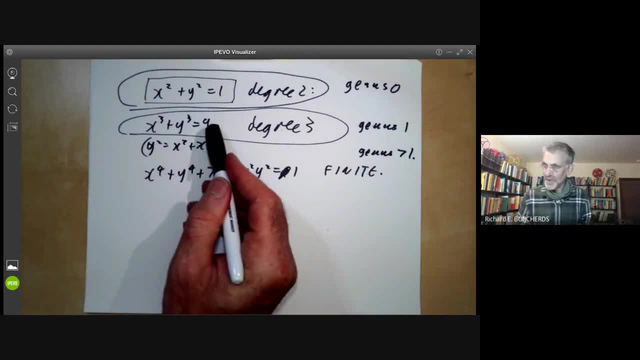 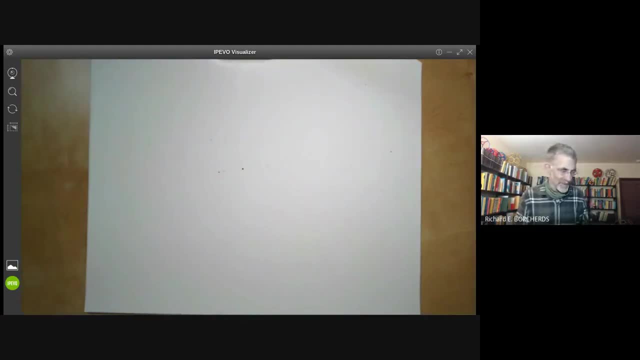 So we've got this really complex number. So we've got this really complex number, So we've got this really weird relation between the topology of a complex curve and the complexity of the number of points on it. Okay, I think I'll just finish by giving a suggestion for further reading. 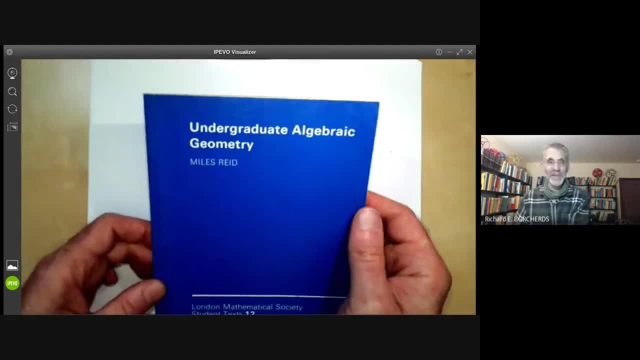 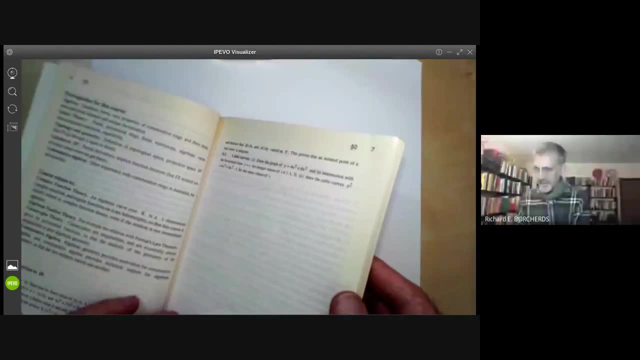 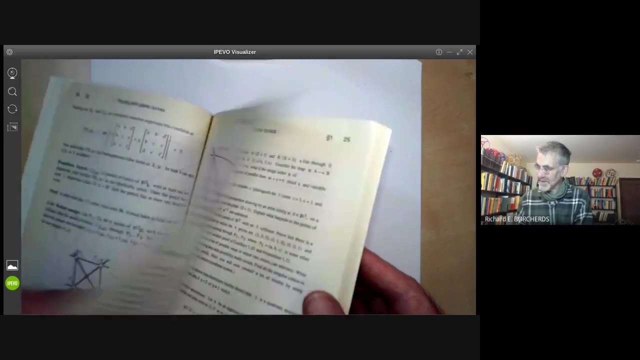 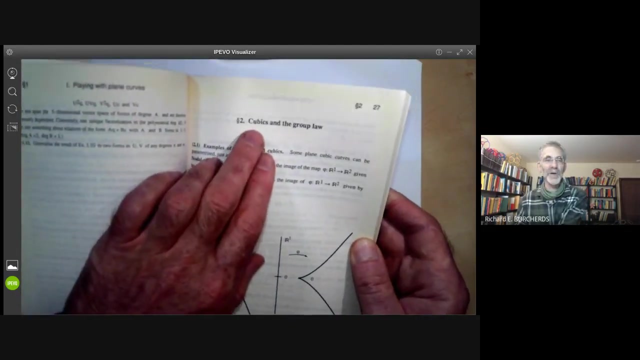 if you want to find out more about this, There's an introductory book called Undergraduate Algebraic Geometry by Miles Reid, and the early chapter on it explains this method of generating rational points on cubics. So here chapter two is on cubics and the group law.